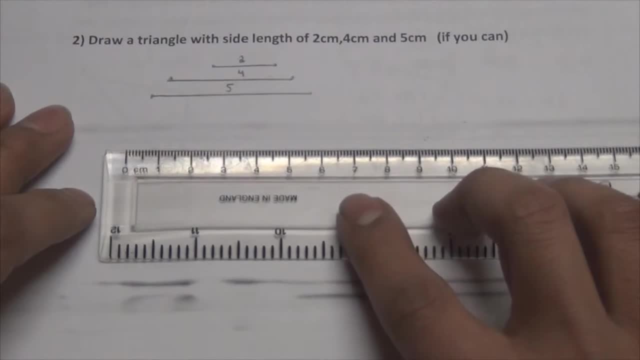 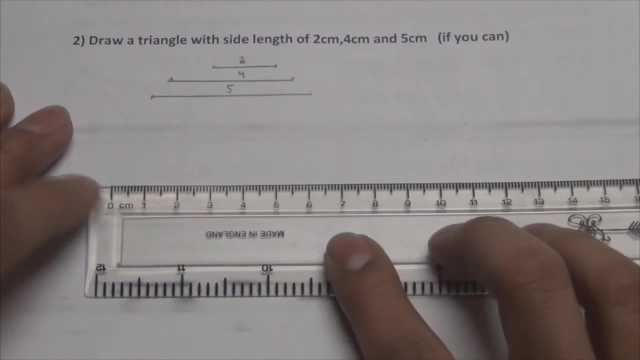 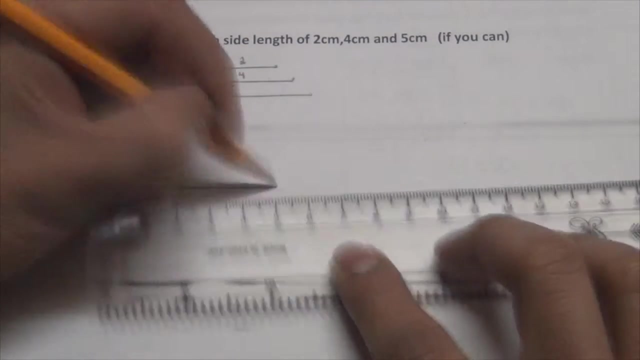 Now you really don't need the ruler, You could just use the compass, but still So I'm going to draw it around here. Okay, so 5 centimeters is going to be From here to here. Oh my God, I really need to sharpen my pencil. 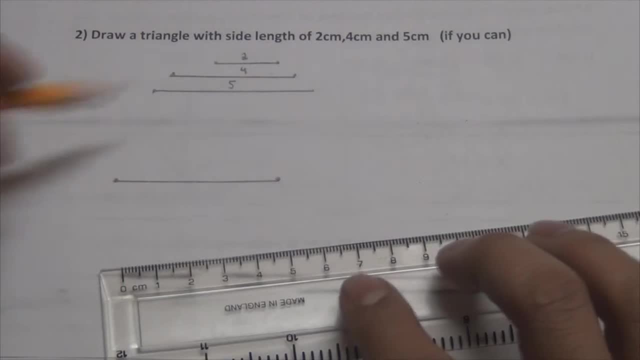 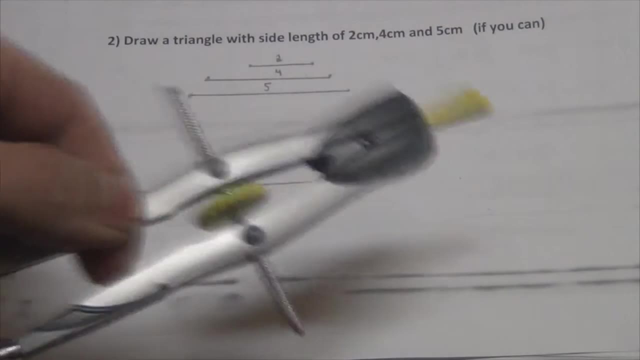 Okay, now I got it All right. now I'm going to be able to do it better. All right, so 5 centimeters. So, from that, guys, what you're going to do is you're going to take the little compass, okay. 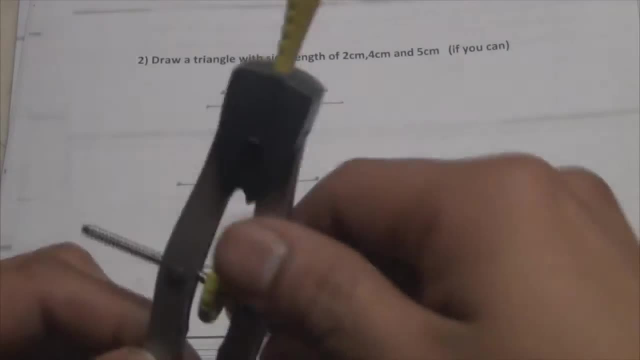 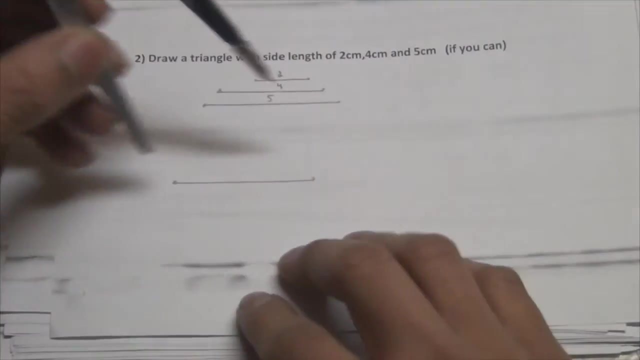 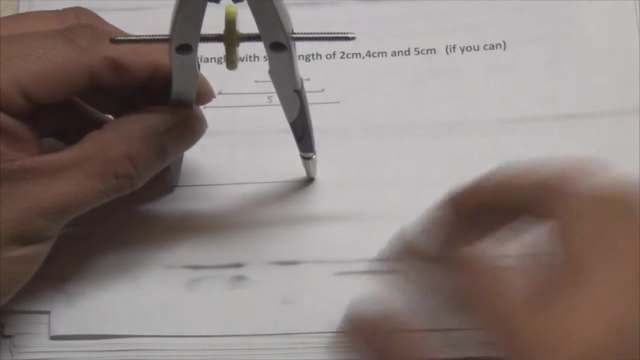 And let me zoom out a little bit. okay, You can still see it, Okay. Okay. So you're going to open the compass, you know adjusting the adjustable wheel to the length of 5 centimeters. So I'm going to put the tip of the compass right here and the other one, ah, almost right here. 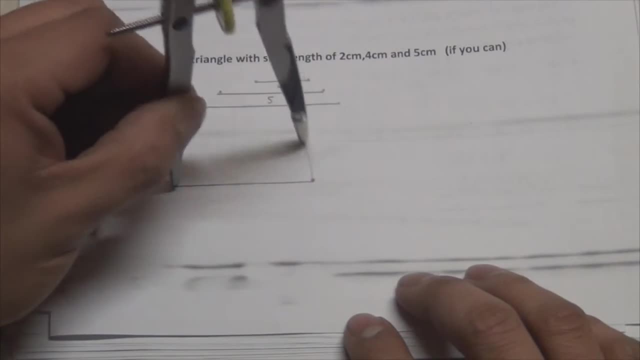 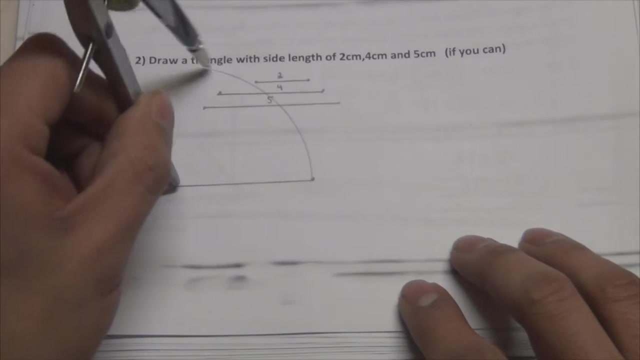 Okay, and what you're going to do is you're going to swing an arc like this, Never mind if it crosses the segments that you already drew. So you do that, Okay. Next, you're going to go to the other, longest segment. 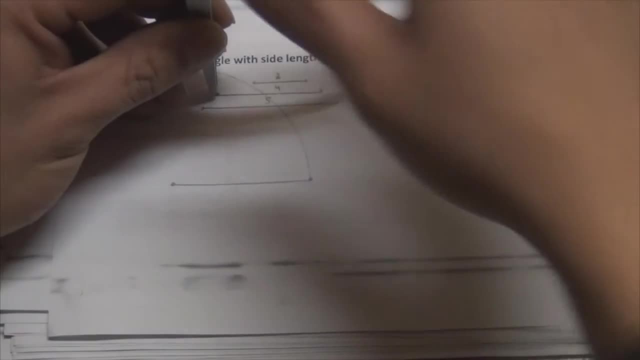 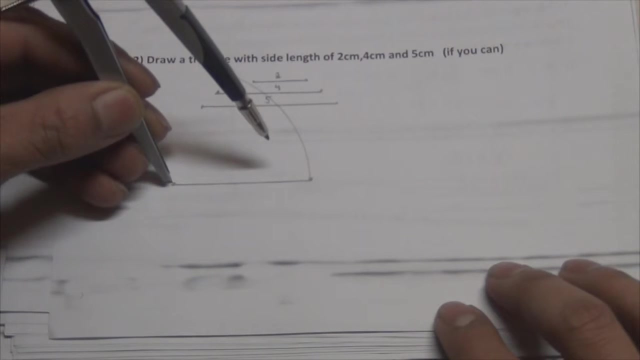 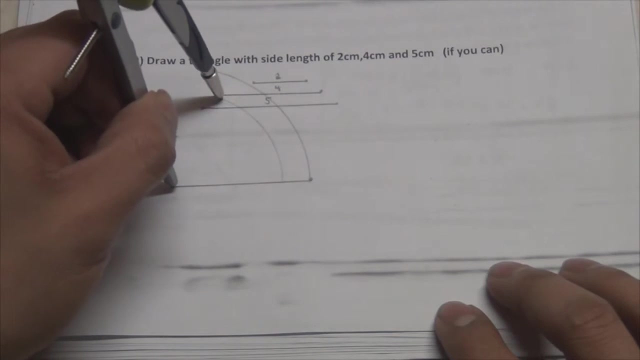 So you're going to put the compass here and you're going to adjust the wheel so it hits the other one- see that- And you're going to repeat the same first step. You're going to put it here and you're going to draw an arc. okay, 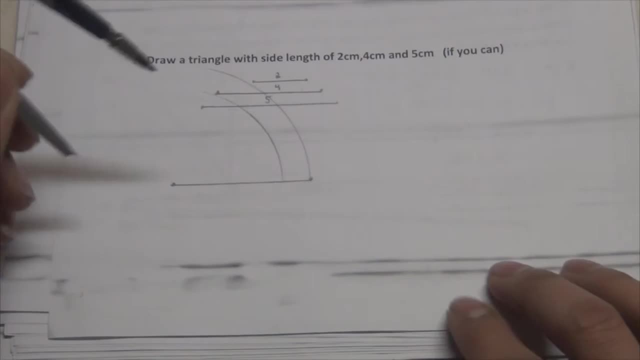 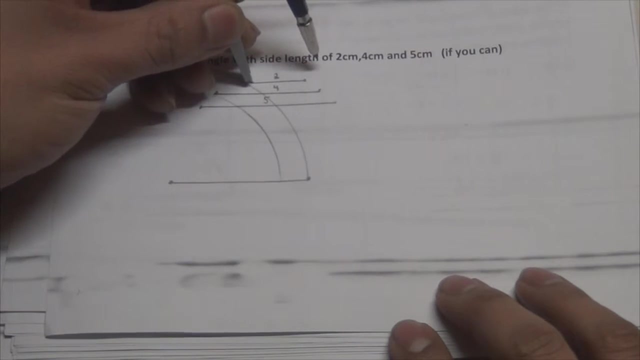 Now, with that arc drawn, then proceed to the next step. The last step is a little different. So you put the compass on the segment that measures 2 centimeters. you adjust it to the other end point like here. okay, see it. 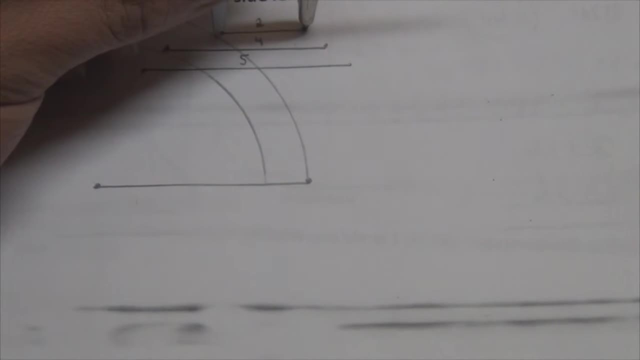 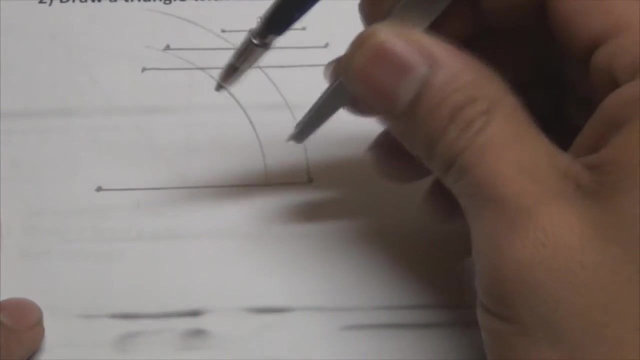 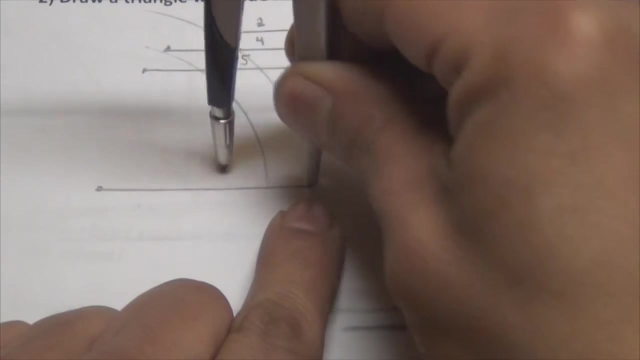 Let me zoom in now. Okay, that's it. You put it right here and now, with that length, you're going to go to the other side of the segment here. okay, here, not here here, And you're going to draw another arc. 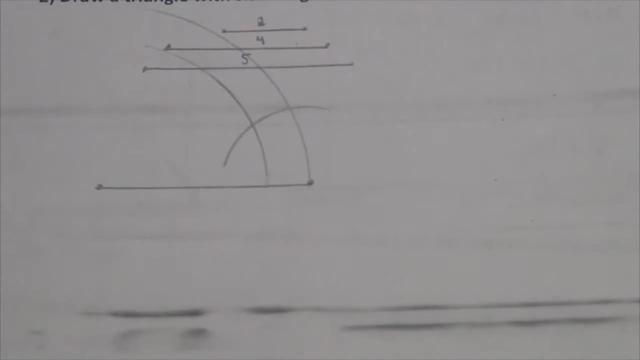 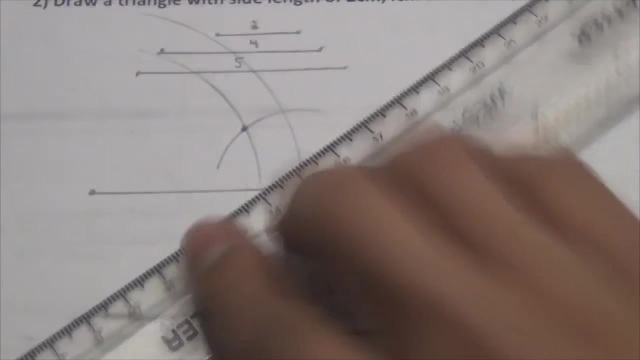 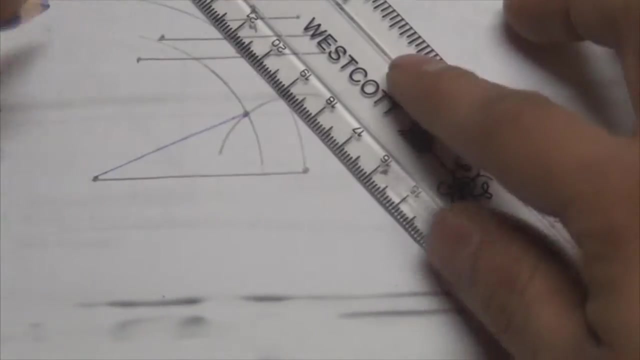 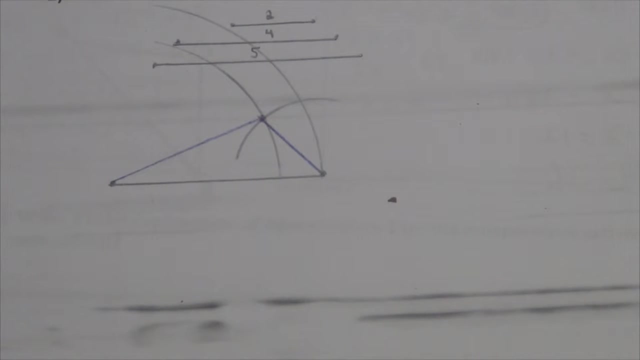 You could do it like that if you want to. Now, what am I concerned about? I'm concerned about this intersection point of the two smallest sides, And now all you got to do is connect the sides, And this is how you draw a triangle with a given length. 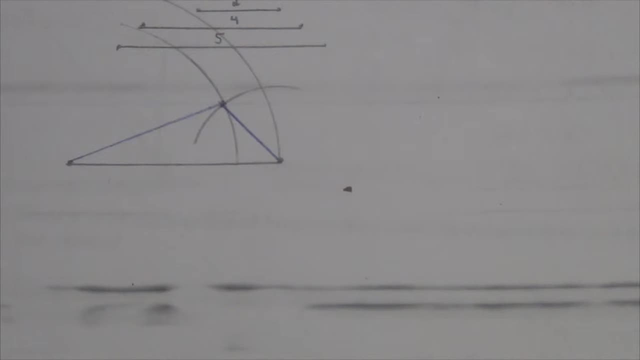 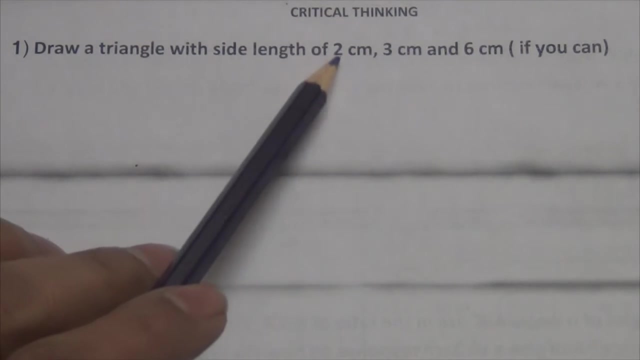 All right then. Now you're going to go to the other side. You saw my triangle. I want you to try using the same technique. I want you to try. why is it blurry? Now I want you to try drawing a triangle with side length of 2 centimeters, 3 centimeters and 6 centimeters. 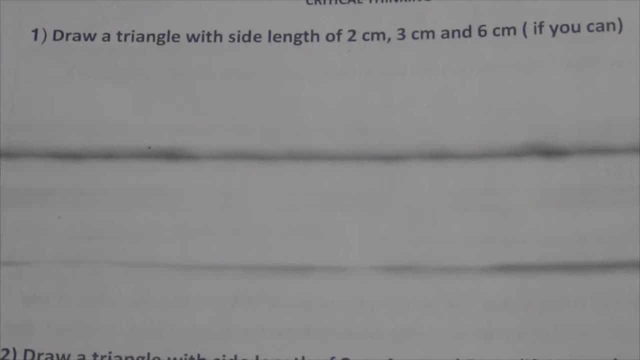 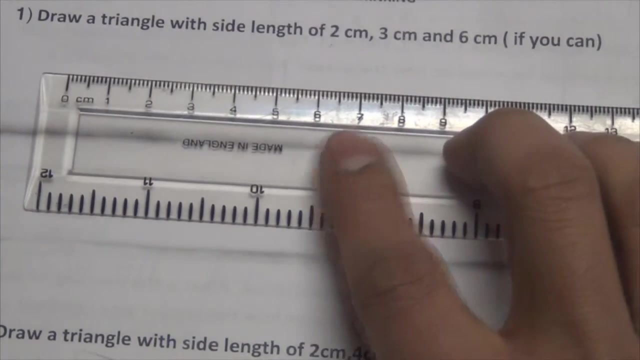 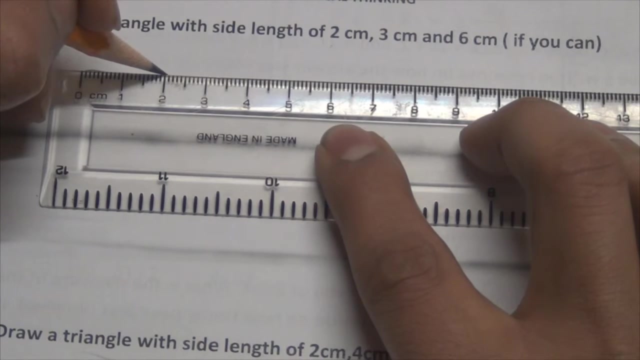 All right, take 2 minutes, do it and reach a conclusion. As soon as you reach a conclusion, boom, raise your hand, Call me, Tell me what your conclusion is and I'll give you one point. So this is going to be my 2 centimeters right here, okay. 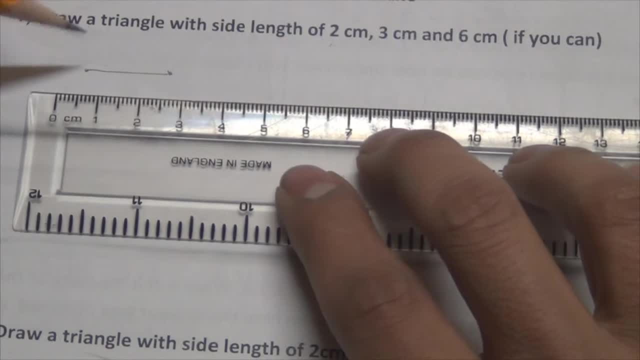 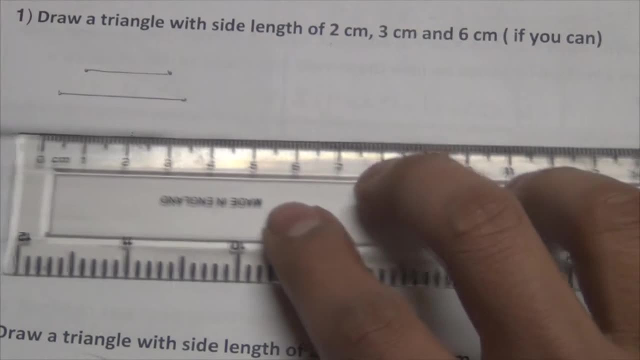 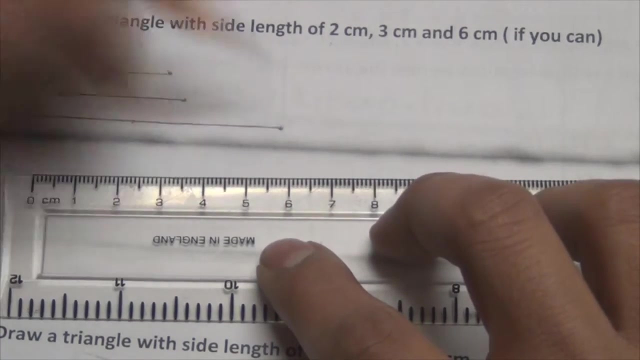 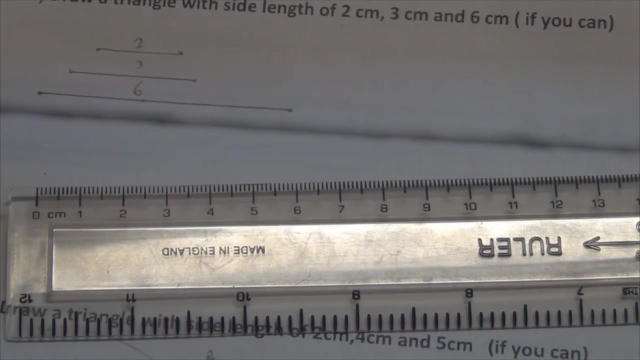 This is going to be my 3 centimeters And this is going to be my 6 centimeters. Okay, so this is 2,, this is 3, and this is 6.. Now, with that, you could just go on to the other side, okay. 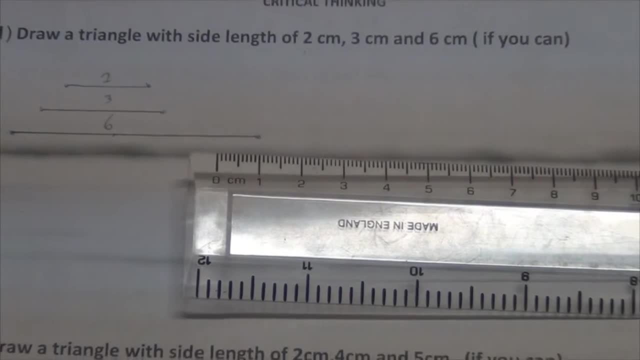 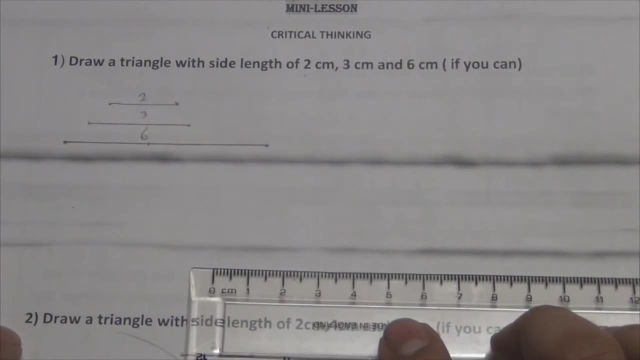 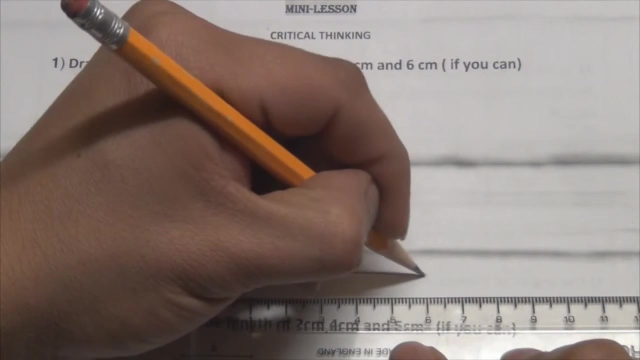 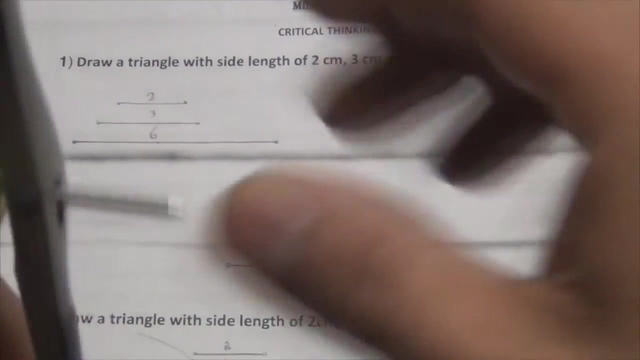 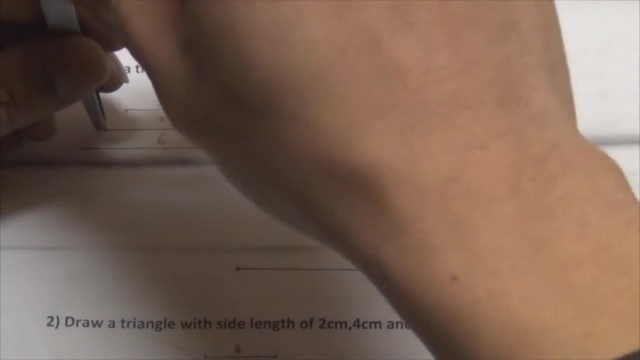 And you draw your 6 centimeters. I'm going to do it over here. 6 centimeters is from here to here. Then remember what you got to do. You're going to the other side? Okay, You adjust the compass to the length of that side. 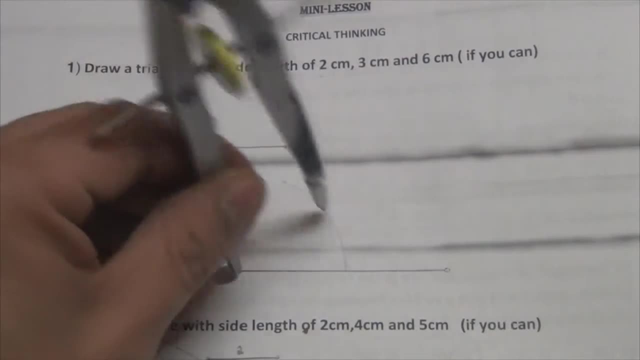 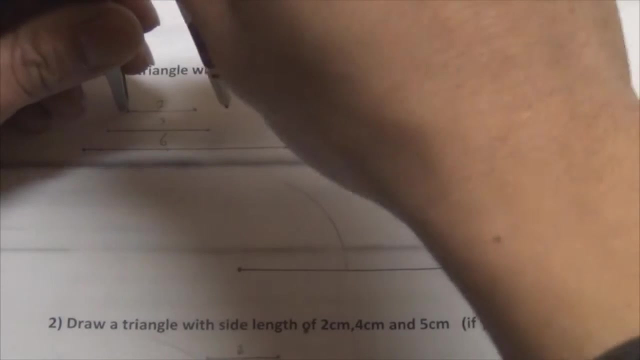 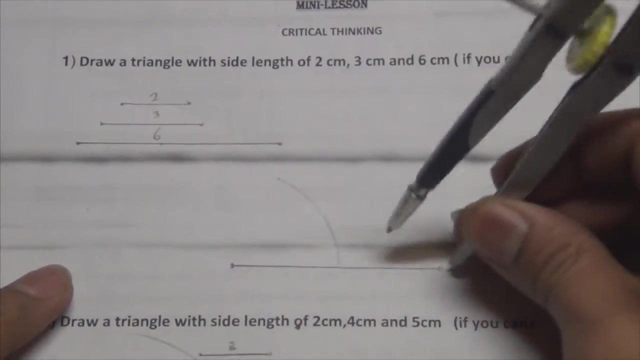 And from here you swing an arc, Then you go on to the other one right here, You adjust the compass, And this time you're going to do it from this side. Okay, Now take 30 seconds to reach your conclusion. 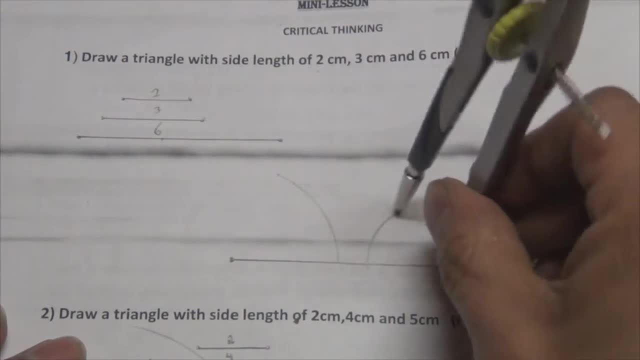 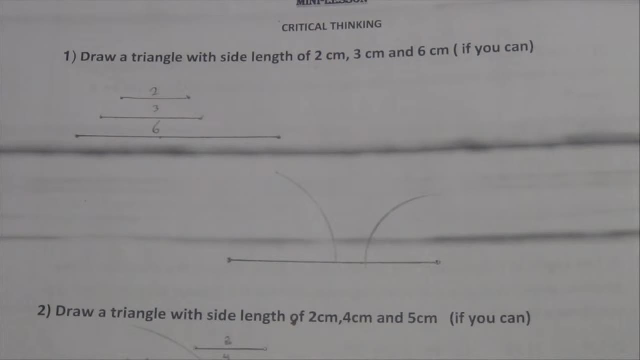 Alright, If you got it, you got it, So I'm going to draw the arc. Alright, I got a problem: The 2 arcs don't intersect. Well, hold on a second, They don't intersect, No, So what are you talking about? 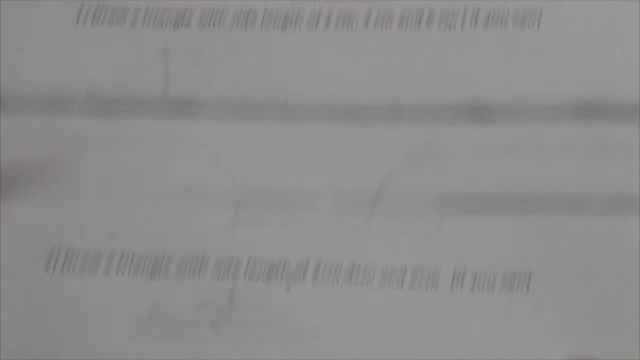 Well, look at the first problem, Actually, the first problem. you didn't even need this little. the first arc, the longest arc, You only needed the 2 smallest arcs. But look at this: The arcs intersected, So I was able to form a triangle. 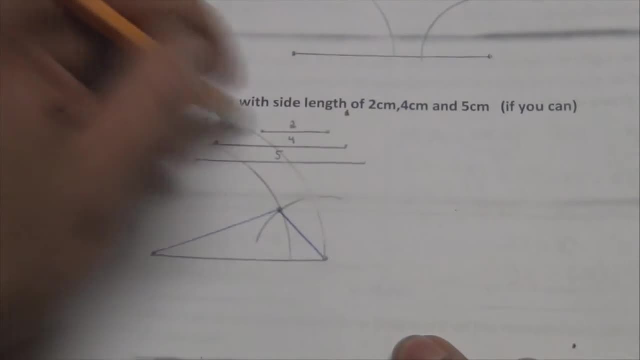 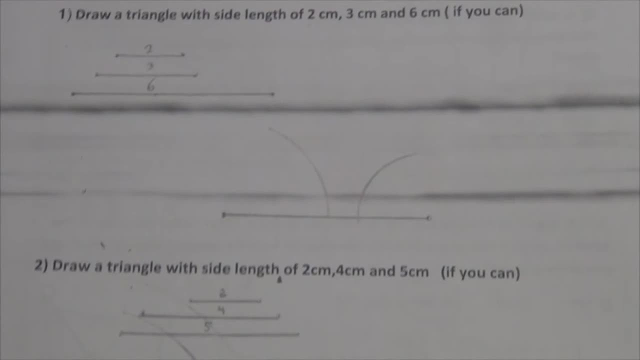 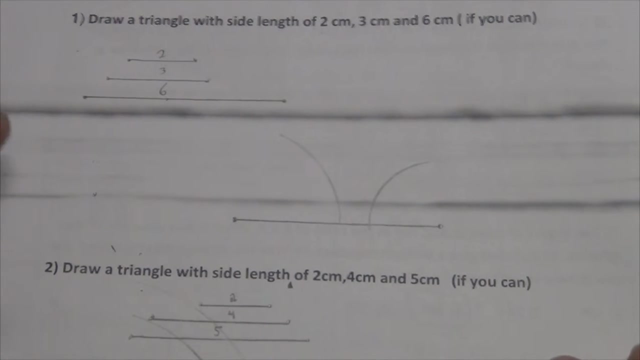 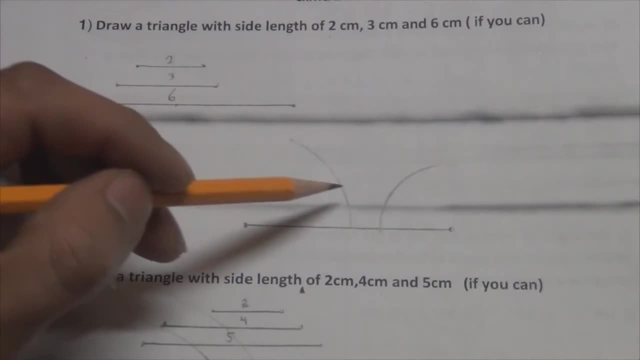 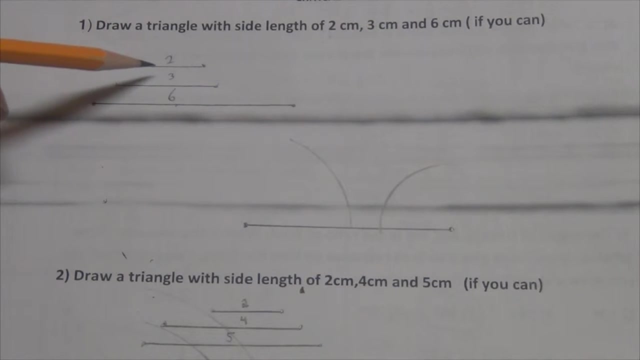 It is set that 2 sides of a triangle. when you add the 2 sides, the length of the 2 sides of a triangle, that length must be greater than a third side, Any 2 sides, any sum of the 2 sides, must be greater than the third side. 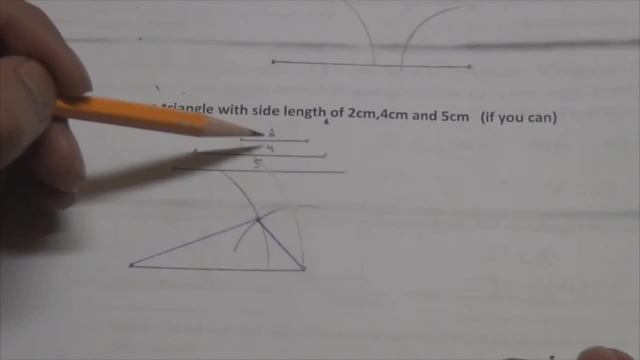 So let us look at the second problem right here and let's see if it's true: 2 plus 4 is 6.. Is that greater than 5?? Yes, Okay, 5 plus 4.. is that greater than 2? yes, what was the other one? 2 plus 5 is 7. is that greater? 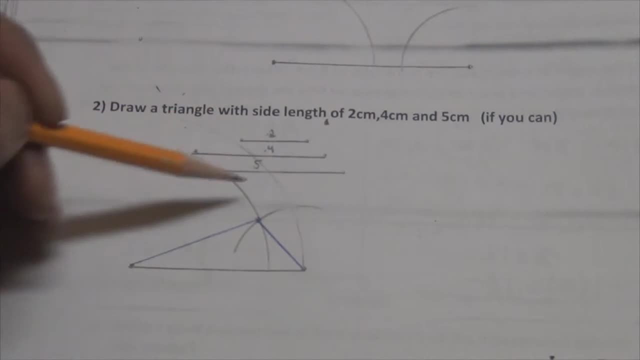 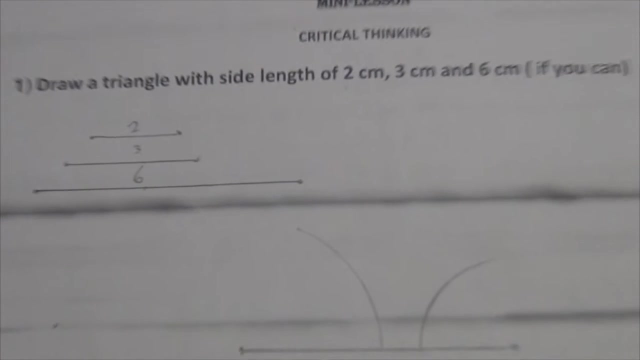 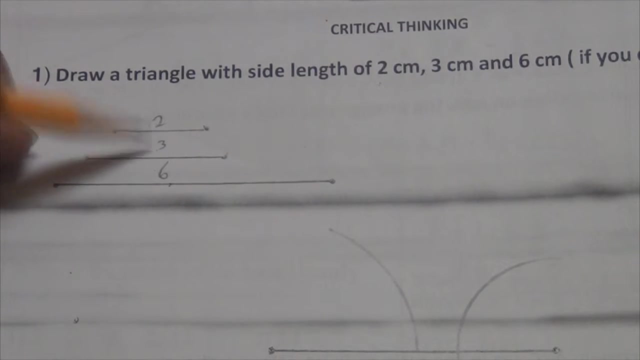 than 4. yes, so that's why this was able to be a triangle now here, if you look at it closer. why is that we were not able to do to draw a triangle easy? 6 plus 3 is greater than 9. 6 plus 2 is greater than 3, but 3 plus 2 is 5. 3 plus 2 is 5. 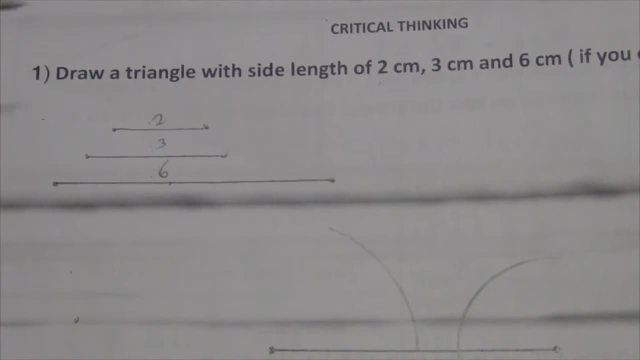 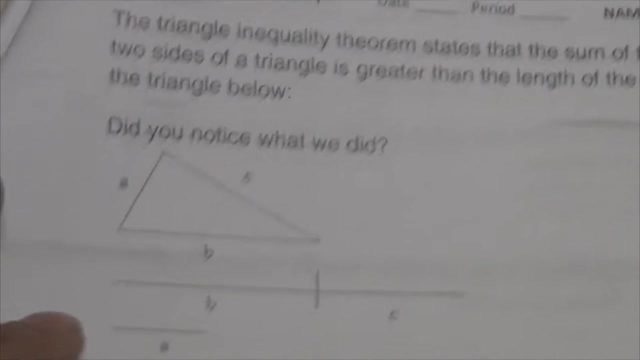 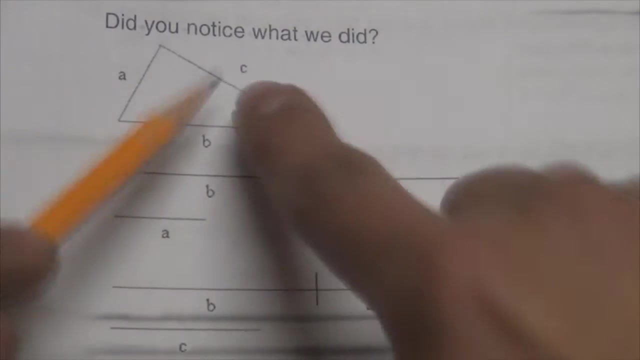 that's not greater than 6. therefore, a triangle cannot be formed. nice, right, that was quick and easy. I told you all right then, so now, here you have your explanation right here. okay, what did you notice? we did, so they, what they did is that they put side B right here and then side C and they expand it. and it was. 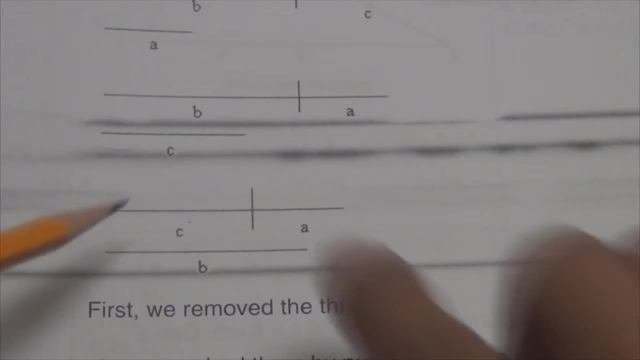 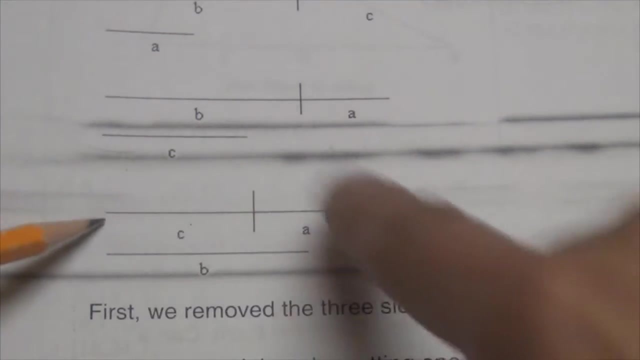 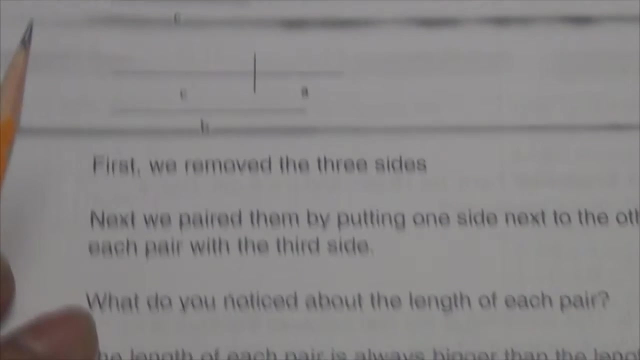 greater than the length of side a, then they did the same thing for side B, and side a was greater than the length of side C, then they did the same thing for side C and side a. see, when you put both lengths together, it was greater than the length of side B. so that's why- okay, that's why we were at. 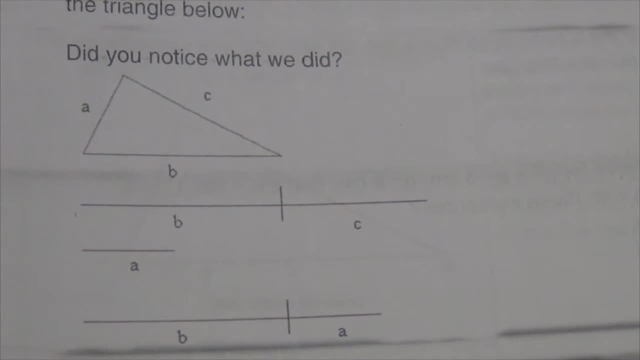 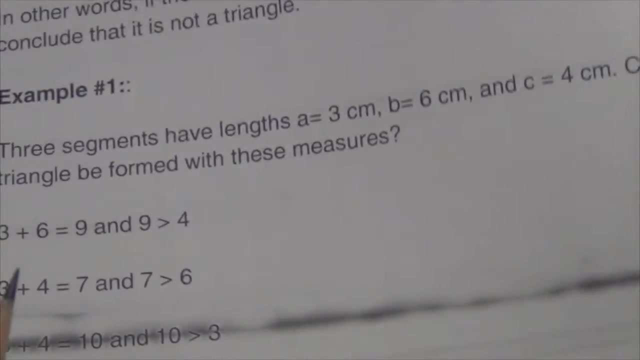 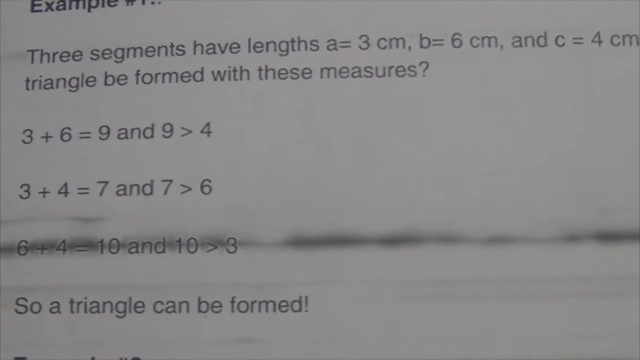 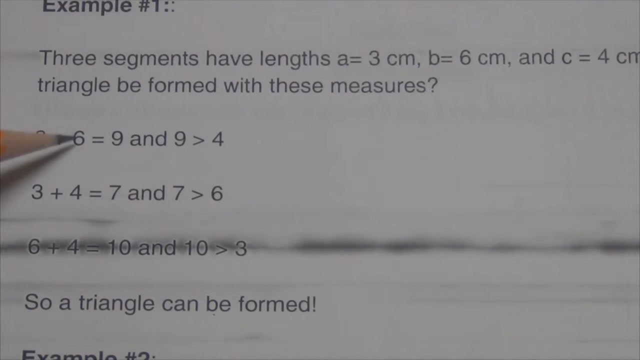 this is able to become a triangle. all right then. so now let's go on to a little problem. so you, it says, three segments have lengths of a equal 3, B equal 6 and C equal 4. so question is: can a triangle be formed by these measures? well, let's say 3, 6 & 9. 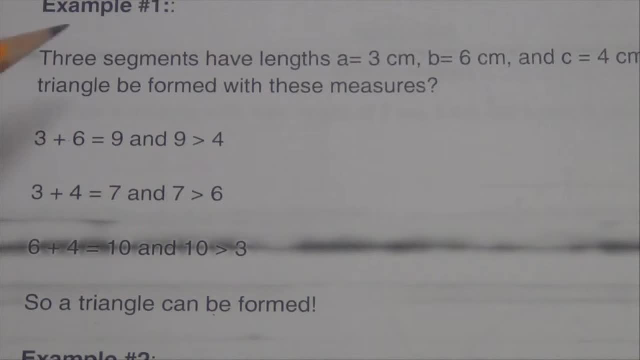 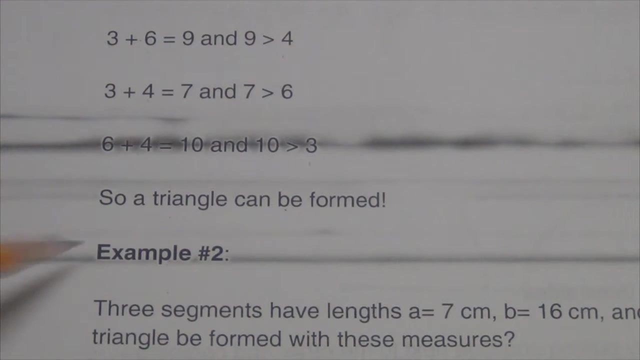 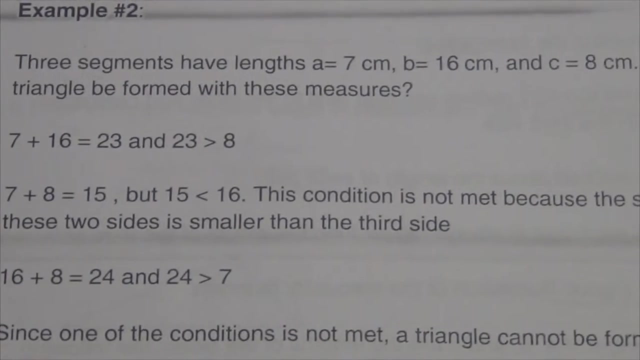 right, so sorry. 3, 6 & 4. is 3 plus 6 greater than 4? yes, is 3 plus 4 greater than 6? yes, is 6 plus 4 greater than 3? yes, so a triangle could be mentioned, Fl, because shouldn't be formed now? example number two: you got the. 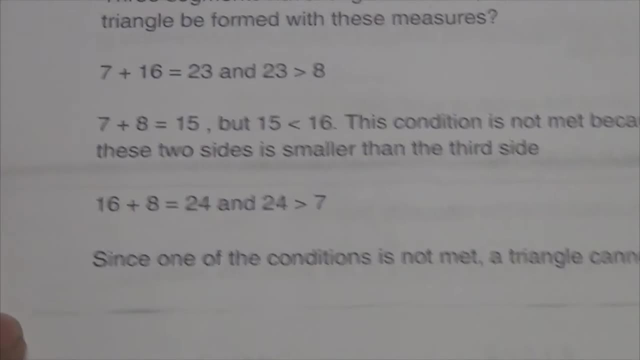 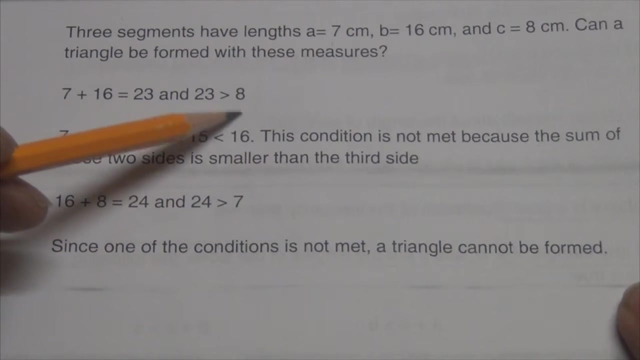 form. now example number two: you got the three lengths. you got 7, 16 & 8. okay, seven, three lengths: you got 7, 16 & 8. okay, seven, sixteen and eight. so let's start working with this. let me zoom out a little bit. okay, so seven plus sixteen is 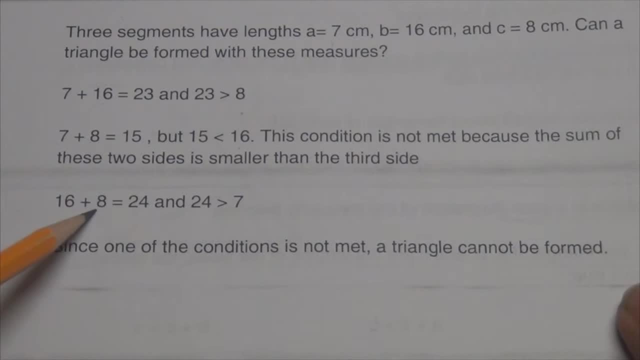 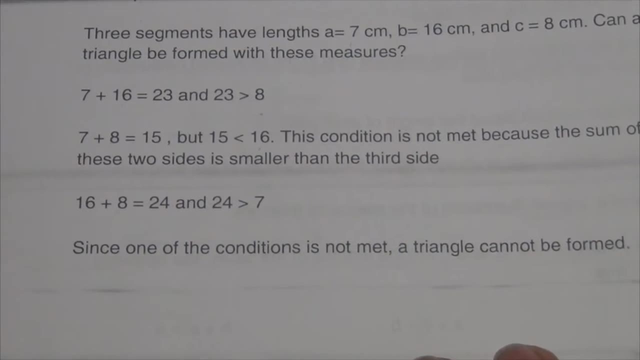 that greater than eight? yes, ok, seven plus eight. is that greater than sixteen? yes, question: sixteen plus eight. wait, hold on a second. which then are you miss? Where did I miss? Oh, my god, sorry, Let's go back here. 7 plus 8 is 15.. Is 15? 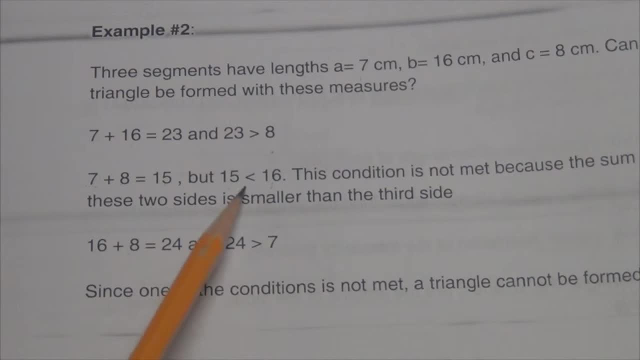 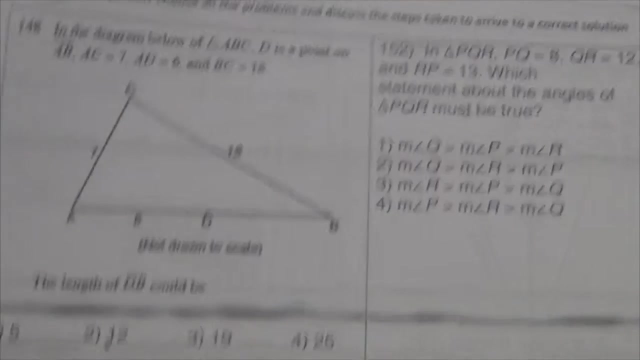 greater than 16?? No, Oh. so guess what? This condition is not met because of the of these two sides. The sum of these two sides is smaller than the third side, So a triangle cannot be formed. Alright, let's check our understanding and let's. 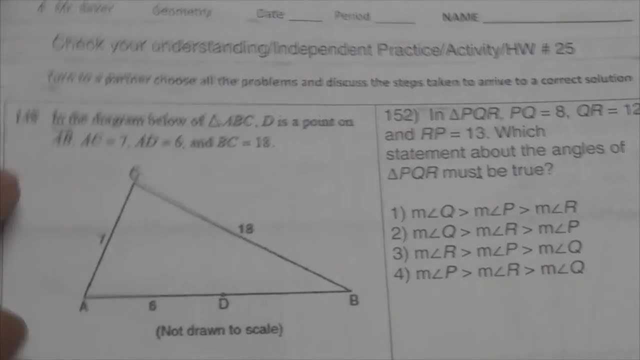 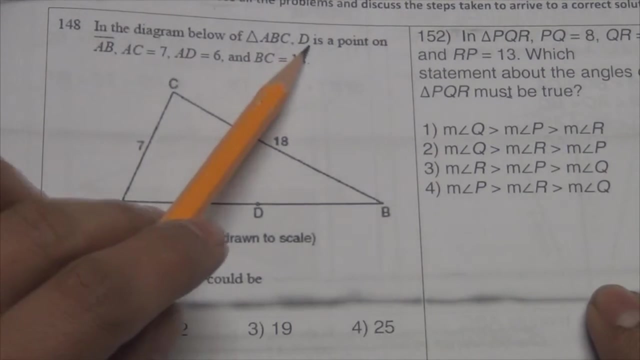 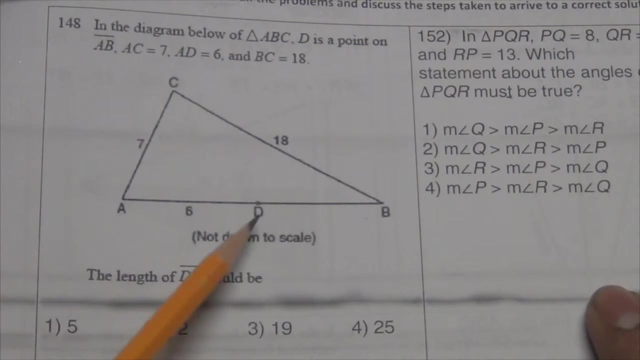 see what's going on. So it says in the diagram below: okay, this is a triangle, D is a point on AB. okay, And they give us the length of each side. They don't give us. this Question is the length of DB could be. So they want this length. I'm. 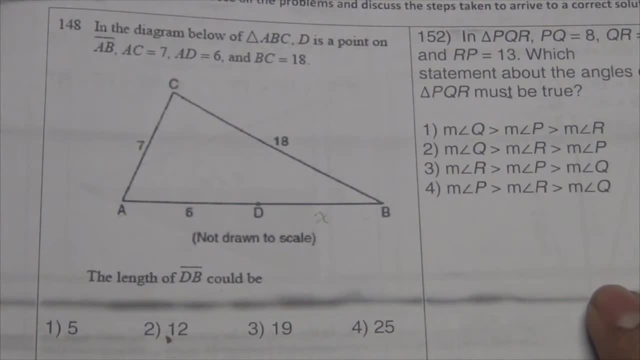 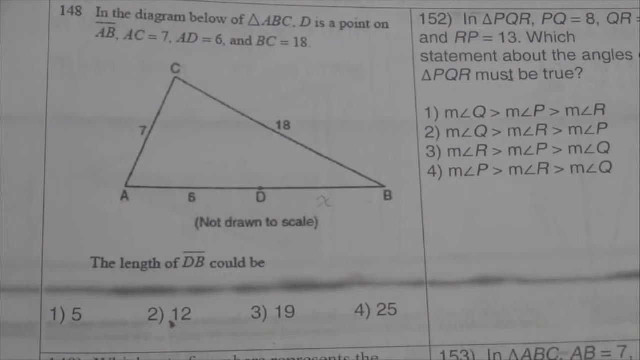 going to call this length X, or I could call it a box, or I could call it N, I'll call it whatever. I need to know what this length is. Alright, so you got choices. If the length of this X was 5, then the length of 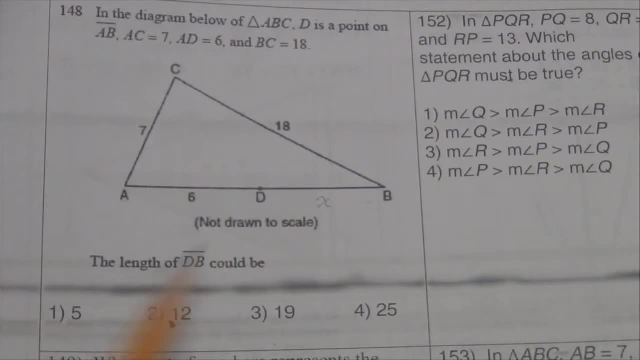 AB would be 11.. So let's try that. 11 plus 7 is 18.. This, is it greater than 18?? No, So this cannot be the length of DB. Let's try 12.. If this is 12,, this will be. 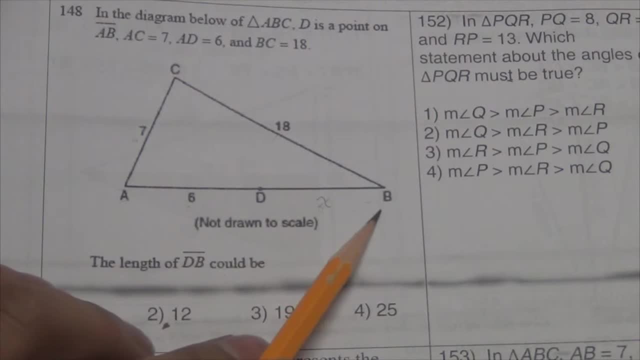 then 12 plus 6 is 18, so ab is 18. so 18 plus 7 greater than 18- yes. 7 plus 18 greater than 18- yes. 18 plus 18 greater than 7- yes. so a triangle can be formed right here. 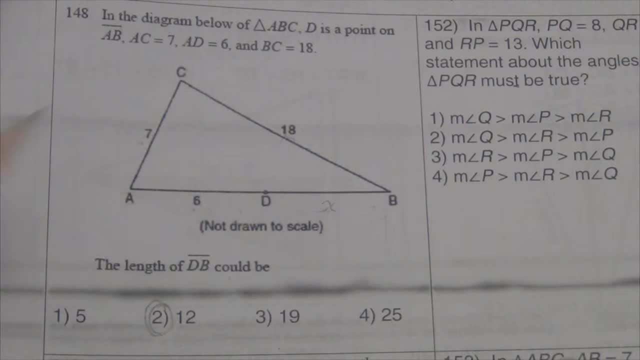 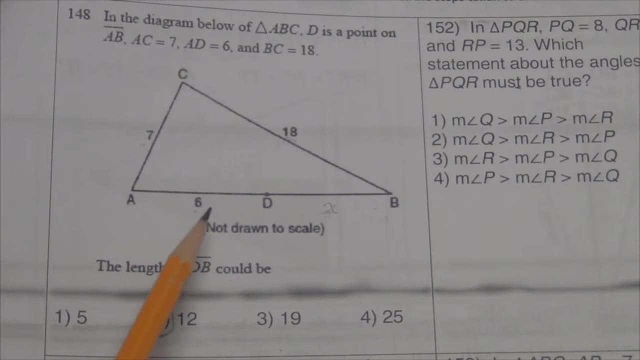 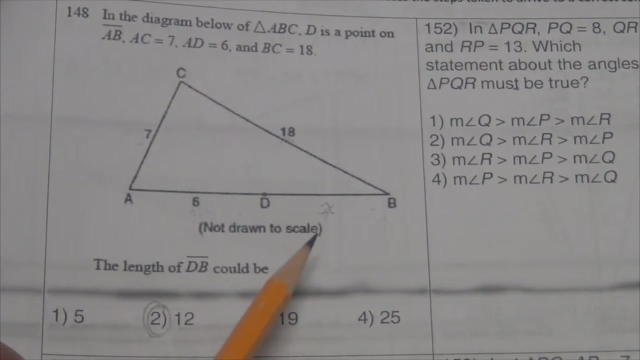 now guess what. some of you might be saying: yeah, but what about 19? and what about 25? sure, let's use 19. if x is 19, 19 plus 6 is 25. hi, hi, how you doing you good, all right. what do you want? play, though? okay, we'll go later. jesus christ, okay, so 19, i said right. 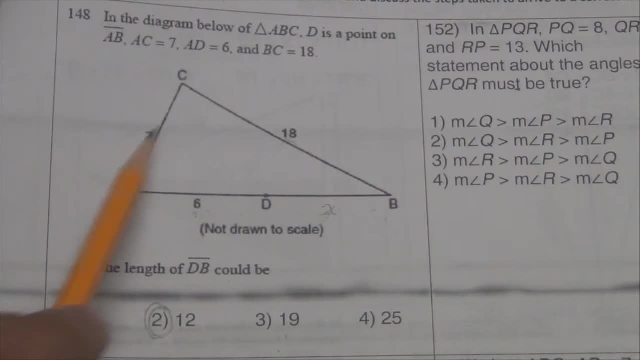 19 plus 6 is 25, but guess what, 7 plus 18 is 25. so this sum: okay, 25 plus 7 is greater than 18. okay, but 18 plus 7 is 25, and that is not greater than 25. 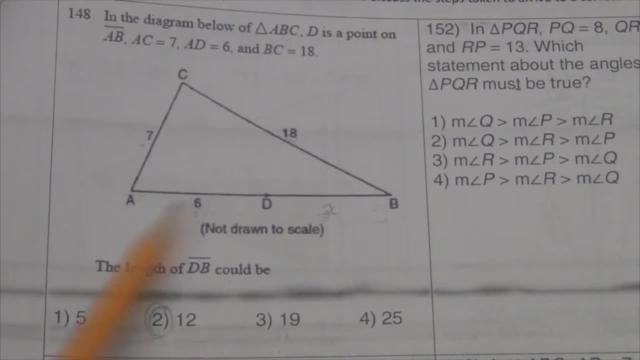 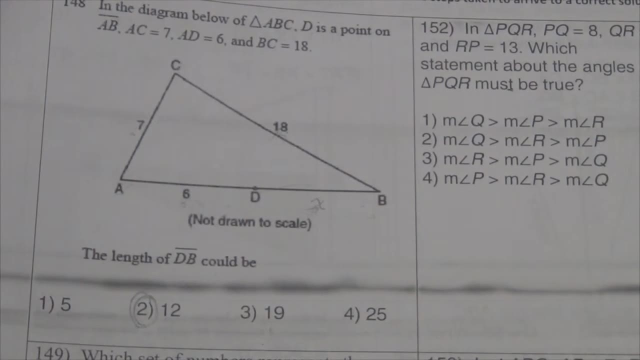 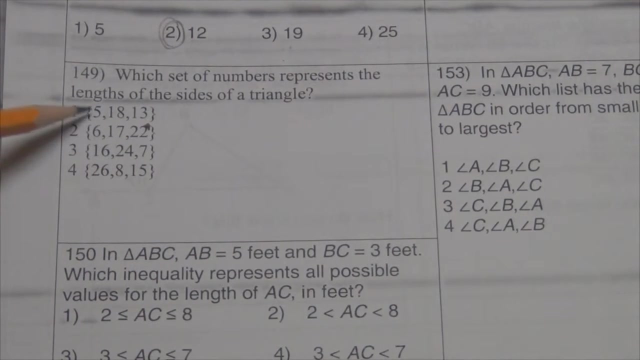 suppose. okay, pretending that this is 12, so then this cannot be a triangle. the same thing goes for 25. use your common sense. all right, let us move on. which of these numbers represents the lengths of the sides of a triangle? well, well, well, Let's see. 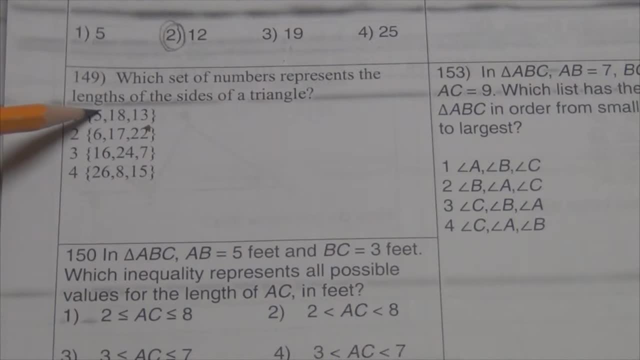 5 plus 18, greater than 13.. Yes, 5 plus 13 is 18.. That's not greater than 18.. So, therefore, this is not a triangle, So this is not the answer. And then 6 plus 22.. 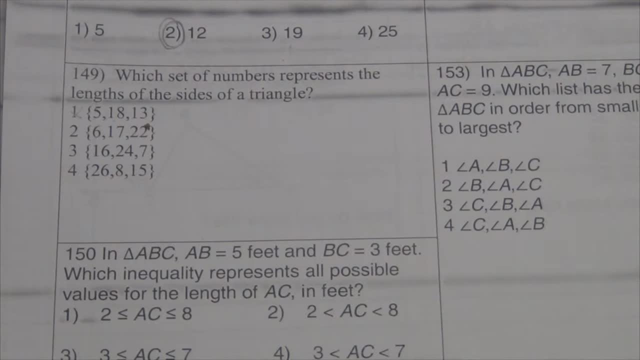 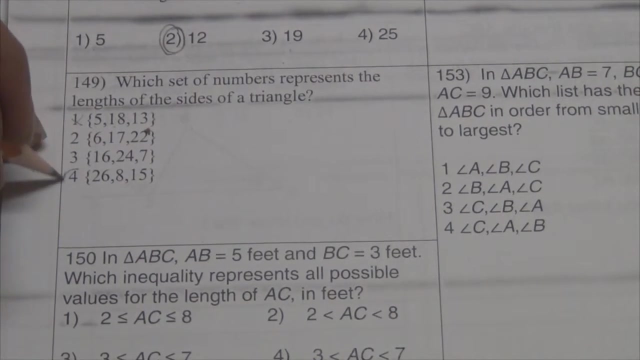 Okay, you get the hang of it. Okay, So take 1 minute or 30 seconds to figure out what the answer is. Okay, All right, so we got our answer. Our answer is 4.. If you raise your hand and you call me, then I'll give you a point. if you gave me the right answer. 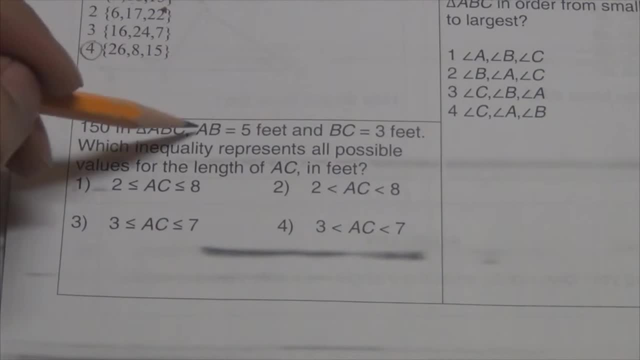 Once again in triangle. ABC, AB is 5,, this is 3.. Which inequality represents all possible values for AC in feet. Okay, All right. so first of all, I cannot work like this. I'm going to have to use a visual, so I'm going to create a triangle. 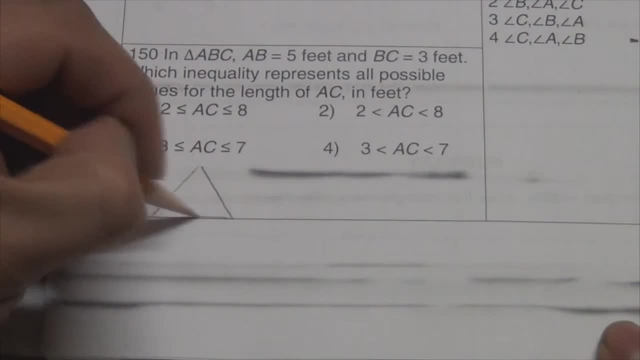 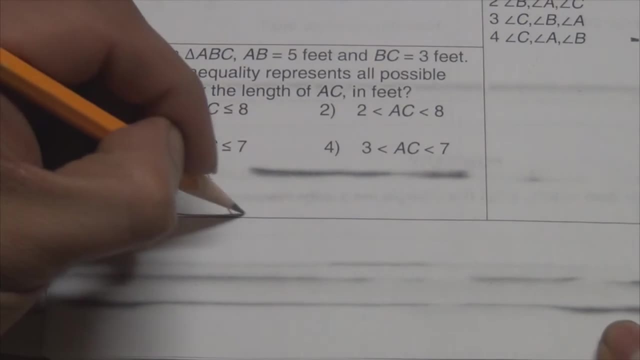 I don't even need the ruler, I'm just going to do a triangle like this. Okay, So one of the sides. okay, in triangle, ABC, so let me call this ABC. Okay, So AB is 5.. So AB side, AB is 5.. 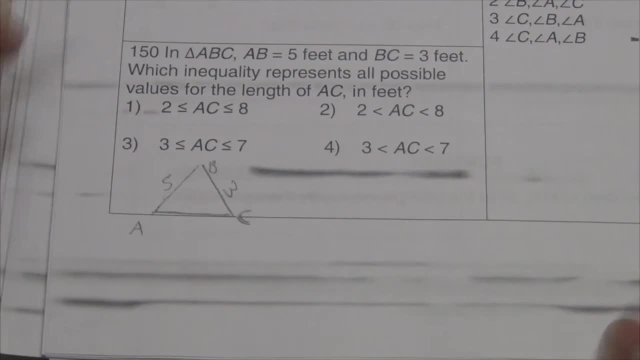 Okay, BC is 3.. Okay, So now possible values for AC. Sure, What do I know? I know that 5 plus 3 must be greater than this. So 5 plus 3 is 8. Okay. 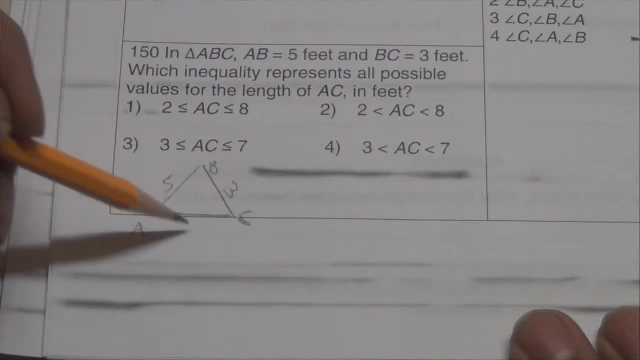 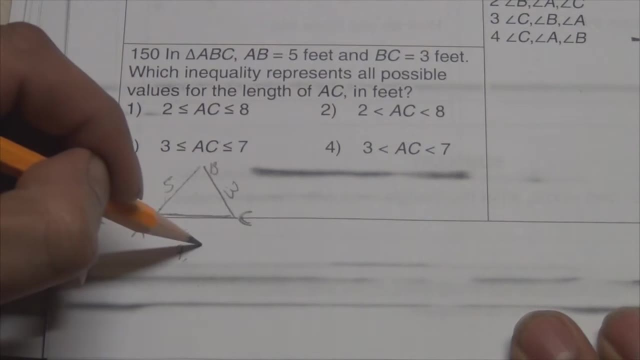 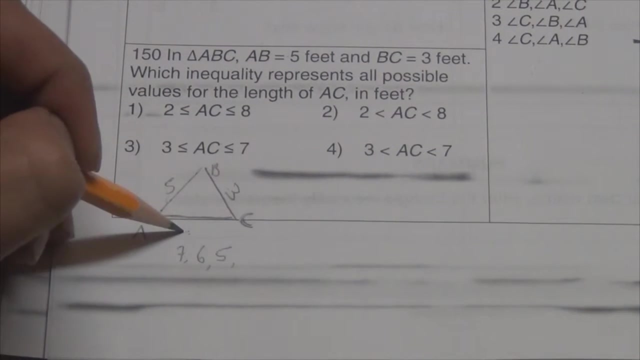 So what are the possible values here? Okay, it could be 7.. It could be 6.. It could be 5.. Can it be 4?? Well, let's see, 4 plus this is 7.. Then this: yes. 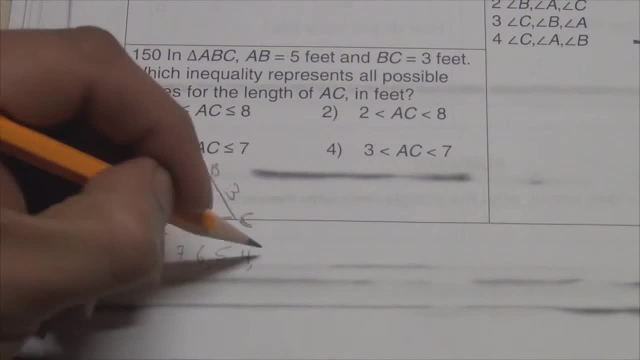 This plus 4 is greater than this. yes, So it could be. It could be 4.. Okay, Can it be 3?? 3 plus 3 is 6.. Greater than this: 3 plus this is 8.. 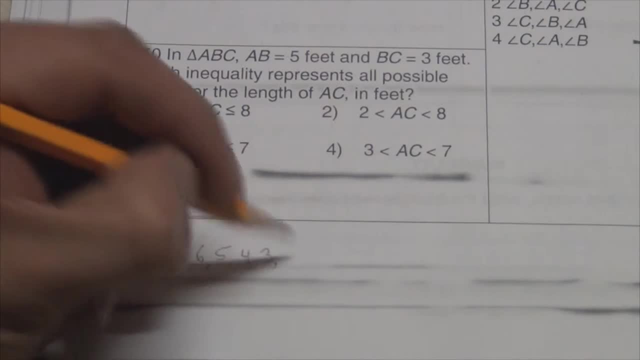 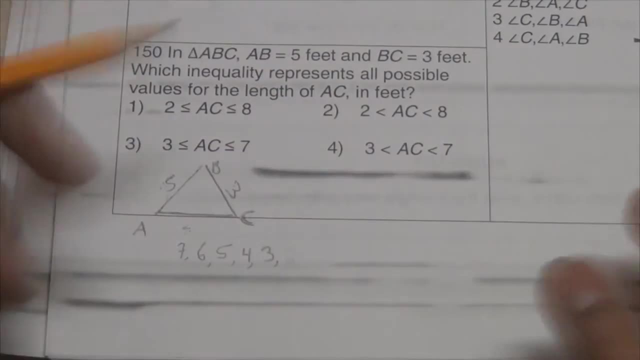 Greater than this. yes, Okay, So now can it be 2?? 2 plus 3 is 5.. Nope, It cannot be 2.. Why? Because if I put 2 over here, 2 plus 3 is 5.. 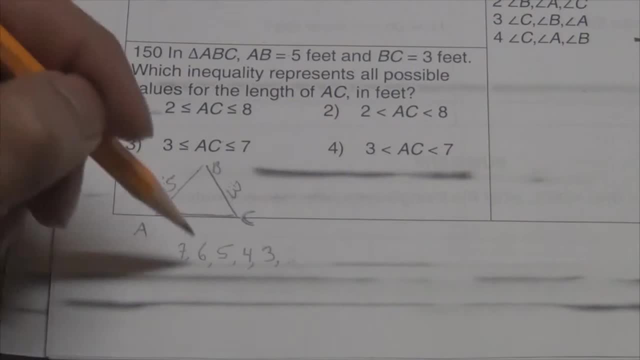 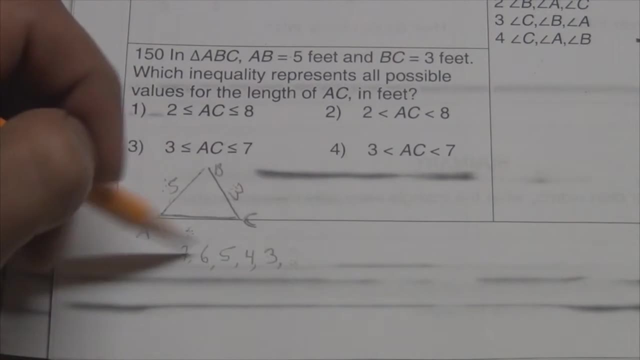 That's not greater than 5.. So forget it All. right then. So the range is from 7, okay till 3.. So does this work? Yes, But is this the answer? No, And why? 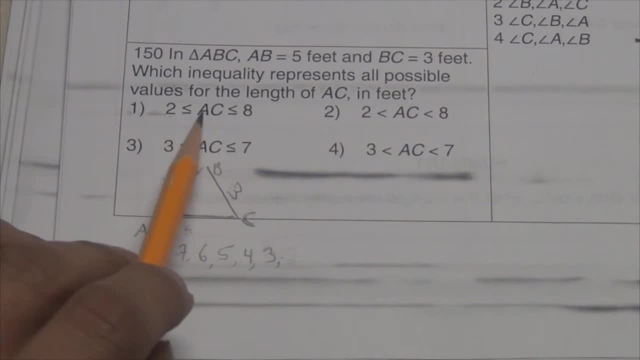 Because we couldn't include the 2 over here. And if you read this, it says: AC is a number between 2 and 8, including 2 because of the or equal to sign, and including 8 because of this or equal to. 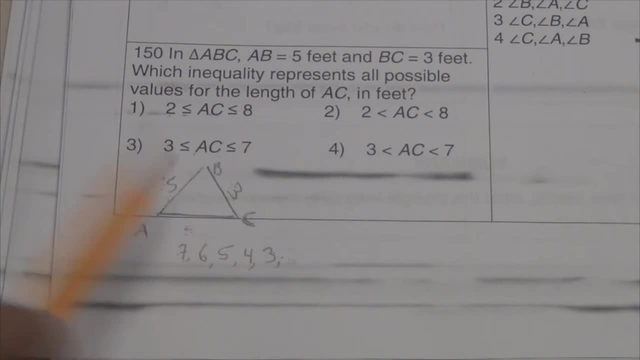 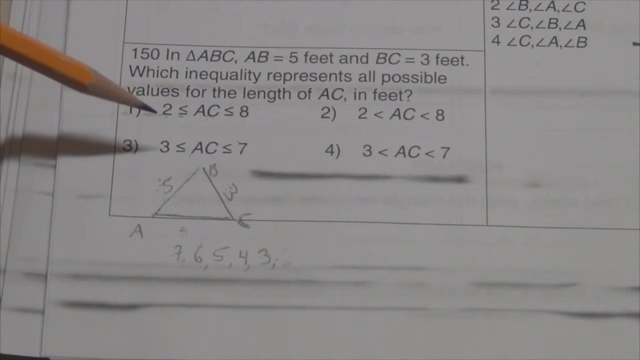 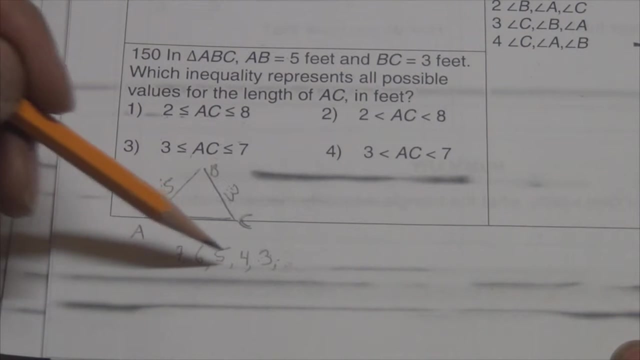 Okay, Okay, AC is between 3 and 7.. Including 3, okay, we have that. Including 7, okay. So this could be one of the answers, But then again, we have a problem And I'm going to tell you: well, it's not really a problem. 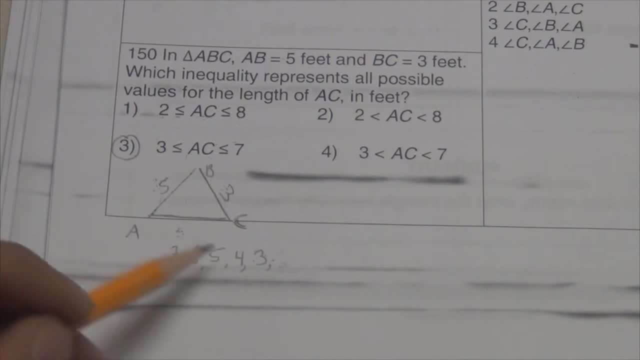 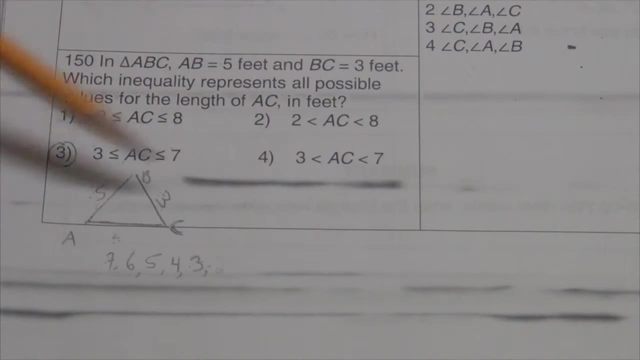 This is one of our answers. okay, because I got the numbers 7 and 3.. Now look at this choice. This choice, my friends, is the same as this one right here. This one says AC. AC is a number between 2 and 8.. 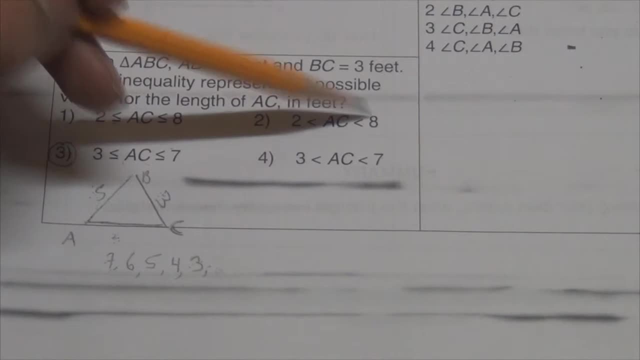 Not including 2 and not including 8.. Well, if you don't include 2, the next number is 3.. If you don't include 8, then the previous number is 7.. Oh gosh, So this could also be an answer. 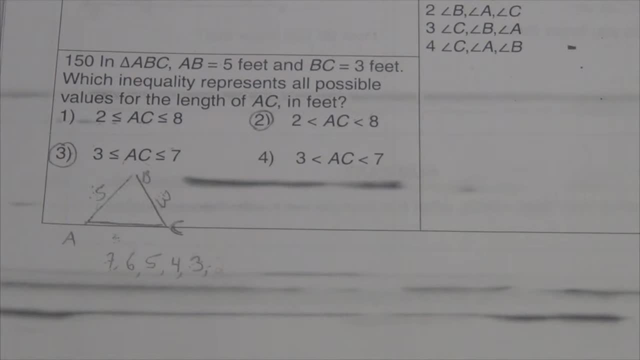 Okay, If you find a discrepancy and you think that cannot be an answer, then you tell me. okay. Now this definitely cannot be an answer because it says that The number is between 3 and 7, not including 3 and not including 7.. 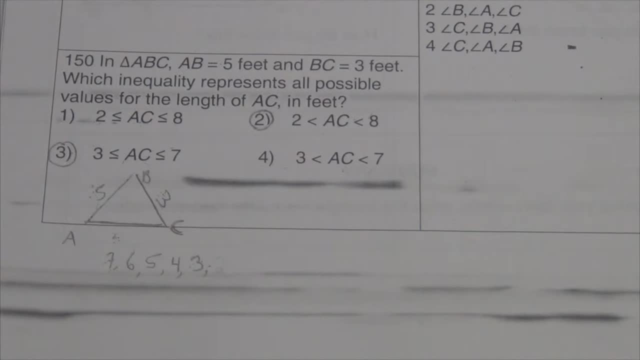 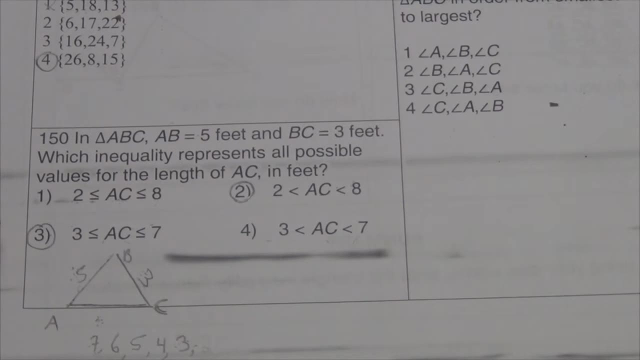 And we already know that 3 and 7 must be included. All right, Good, So we got two choices right there. Now, is it always the case? No, This is a one-of-a-kind question, okay, where you have two choices. 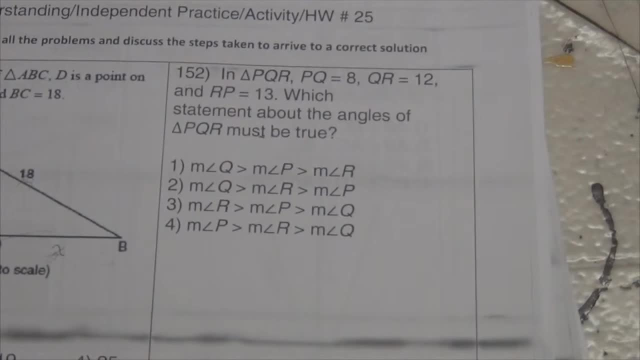 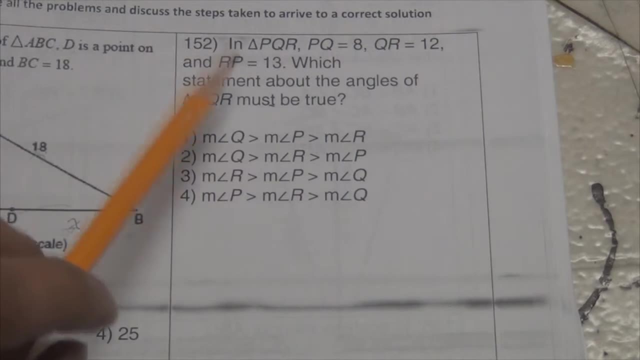 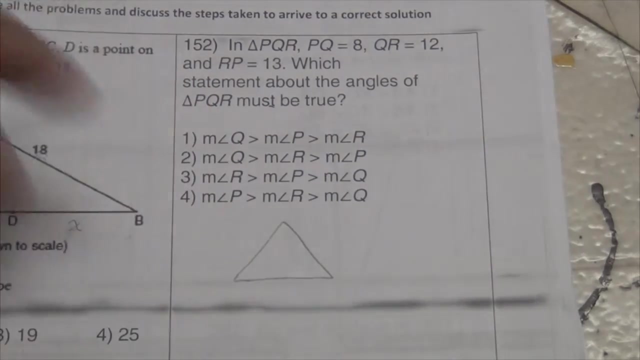 Usually, most of the time, 99% of the time, you're only going to have one choice. All right then. So guess what Let's see In PQR. okay, I need to draw a triangle, Since they're not specifying that this should be a right triangle. 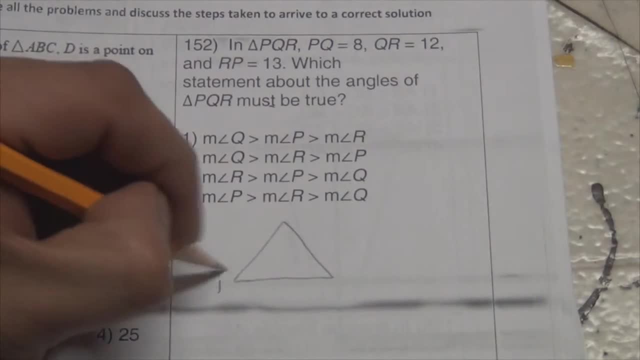 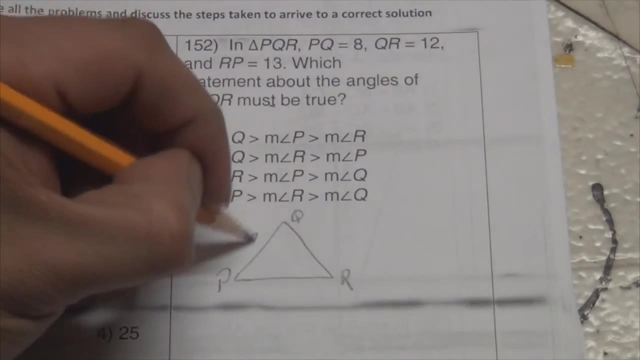 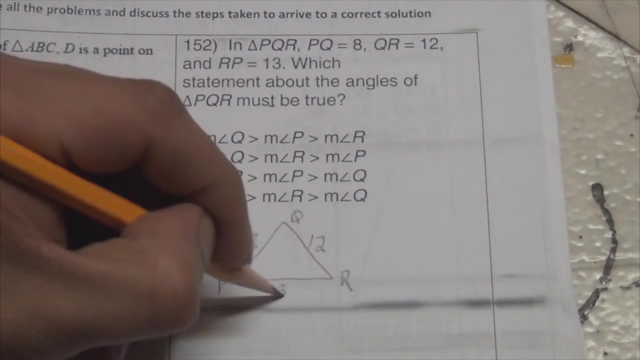 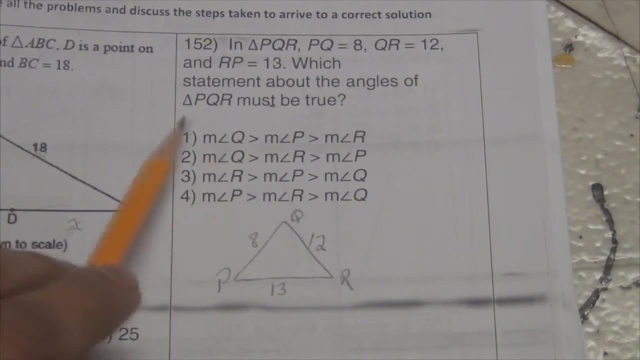 then I don't have to draw a right triangle. So PQR, P-Q-R. Oh okay, PQ is 8.. QR is 12.. RP is 13.. What do they want? Which statement is true? This, sorry, which statement about the angles must be true. 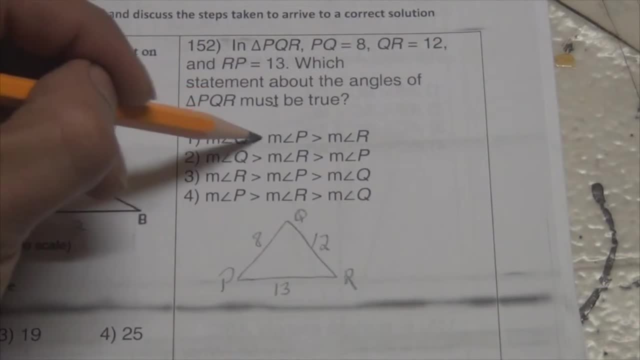 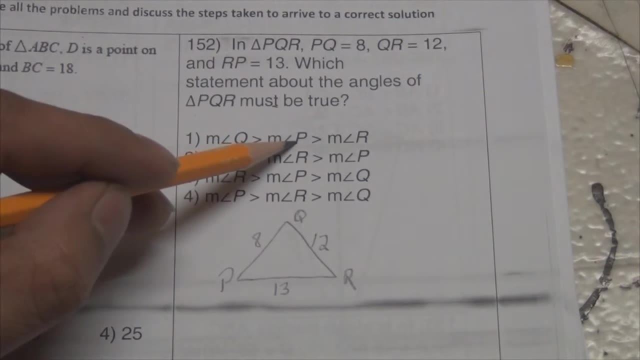 Angles of this triangle must be true. Okay, Notice that these are greater than symbols. That means that the measure of Q must be larger- okay, greater- than the measure of P, And the measure of P must be greater than the measure of R. 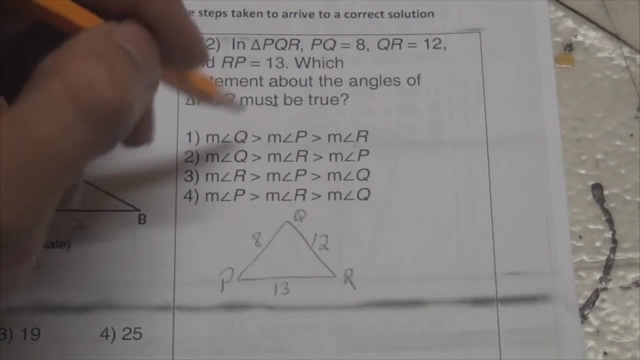 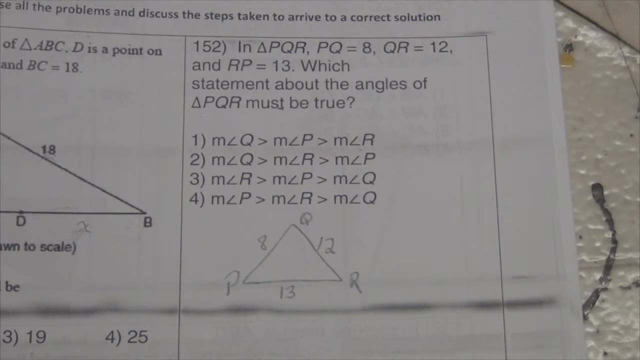 What does that mean? Easy, That we have to arrange the angles from largest to smallest. That's all it says. Okay then, But how am I going to do that? Oh, you forgot, Don't worry, I will tell you right now. 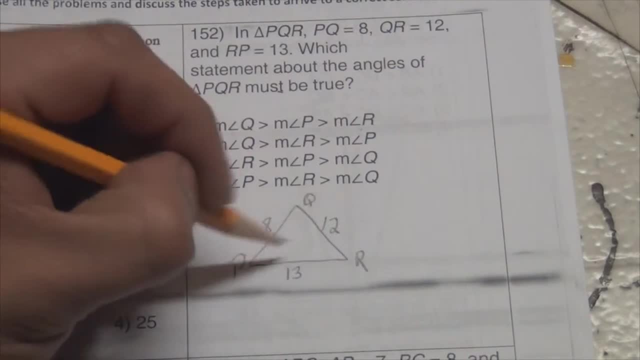 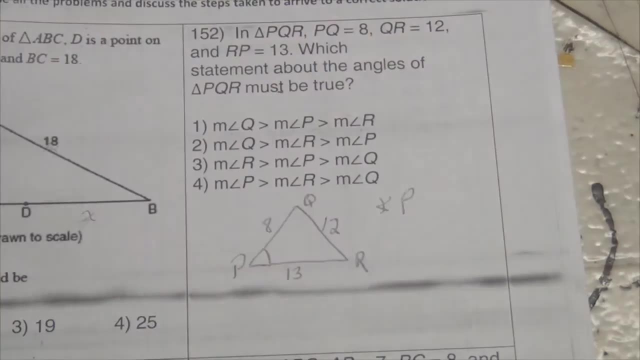 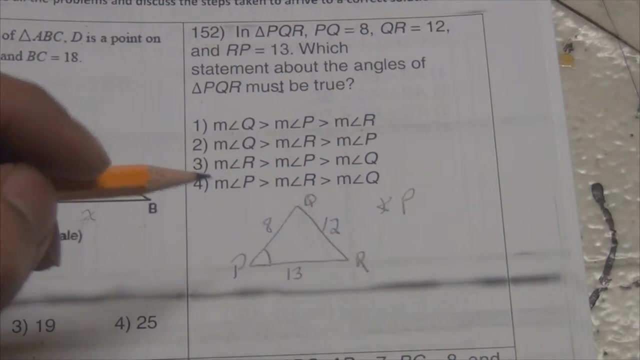 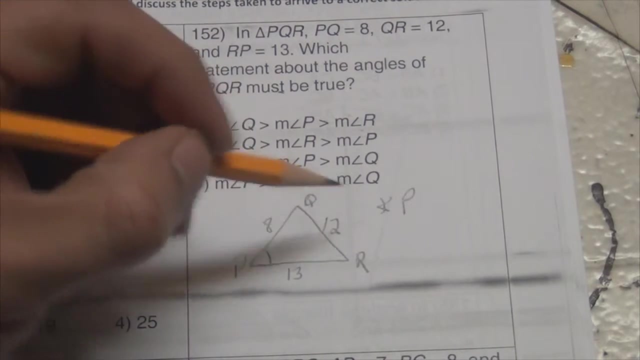 Opposite to the longest side is the largest angle, So the largest angle here is P. Remember, opposite to the smallest side is the smallest sorry, sorry, sorry, sorry. Opposite to the shortest side is the smallest angle, So the smallest angle is R. 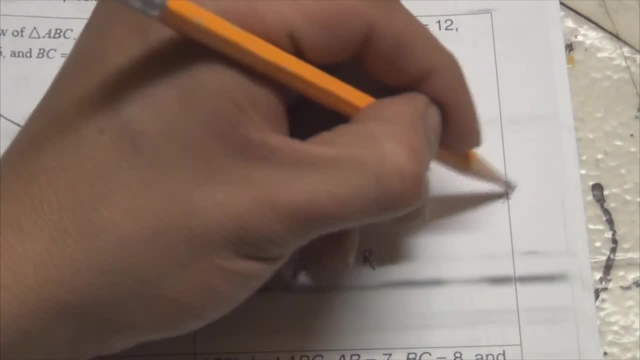 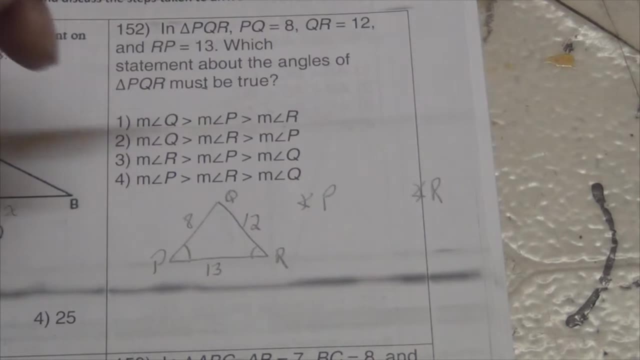 Oh, okay, I get it So R. So what does that mean? That the middle angle must be: wait, hold on a second. How did I get this? Okay, let's go back here. I made a mistake. 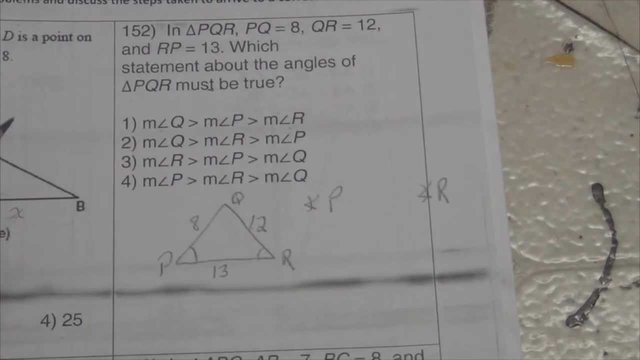 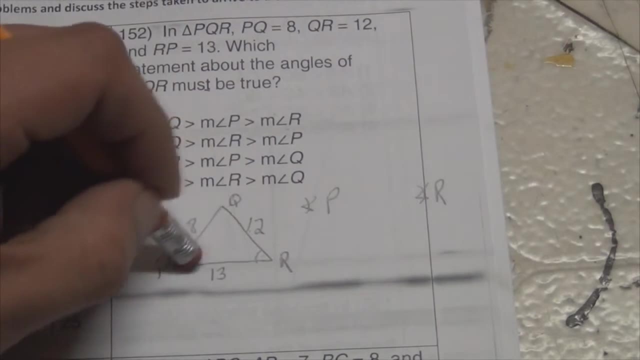 I thought that 12 was the longest side. If you corrected me before I corrected myself, I'm going to give you two points. The longest side is not 12.. The longest side, The longest side, is PR, which is 13.. 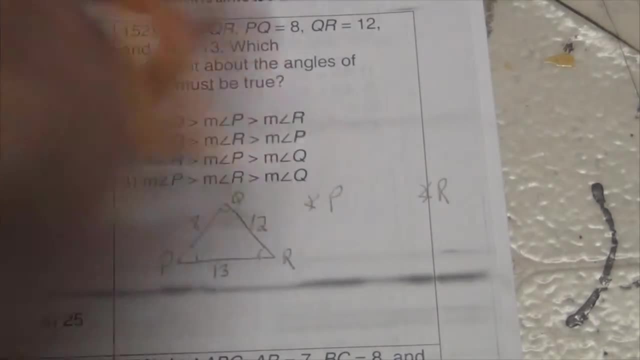 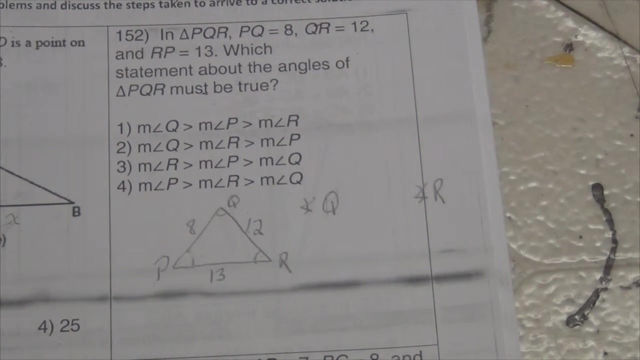 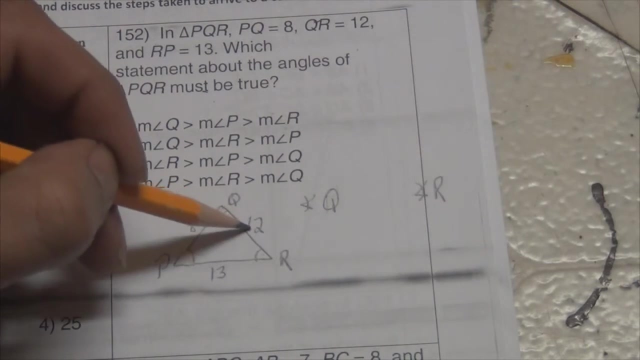 So opposite to 13 is angle Q. Oh, okay, So guess what? The largest angle is angle Q, The smallest, of course, is still angle R And the mid-sized angle is angle P, because that's 12.. 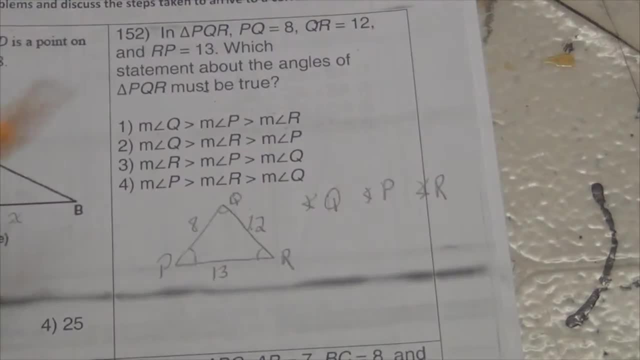 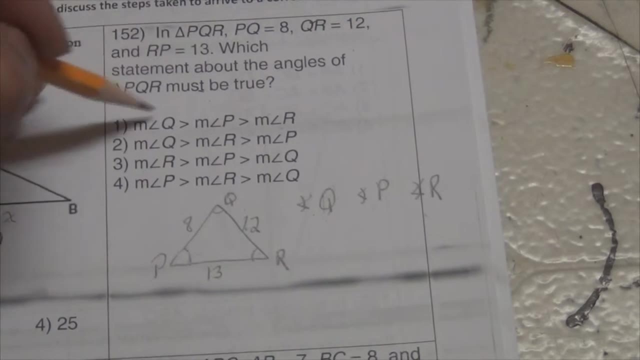 Opposite to 12 is P, So angle P. So I just put them in order from largest to smallest: Q P R, So Q P R. So guess what Choice one is your answer. 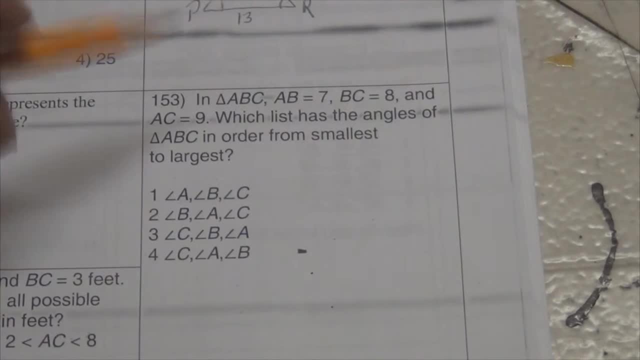 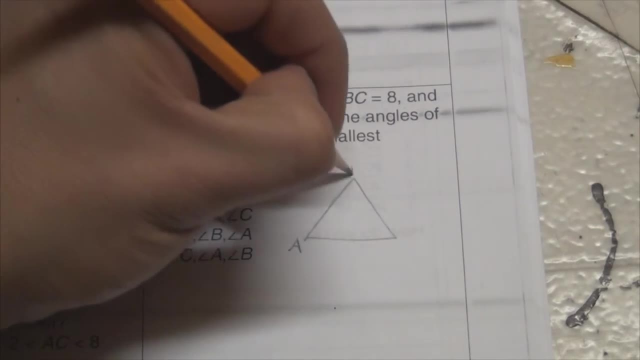 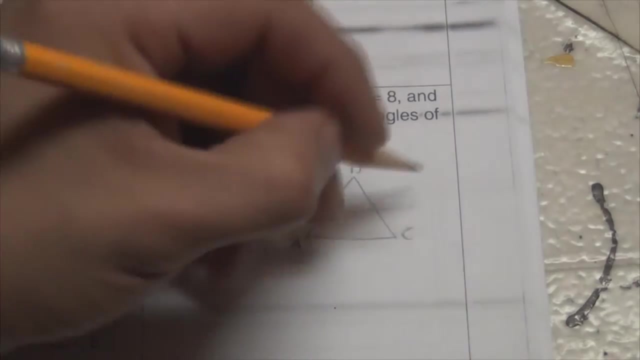 Okay, Let's do this one. It says in triangle: okay, once again I got a triangle. Okay, A, B, C, A B C. So A, B is 7.. B, C is 8.. 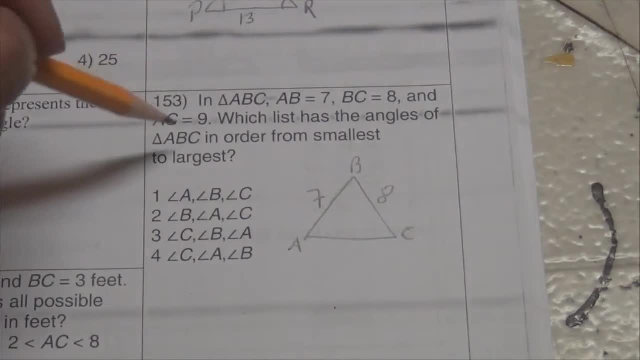 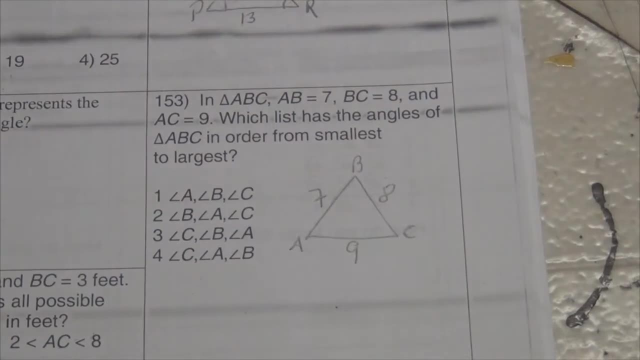 Notice how I label sides. If they were talking about angles, I would go inside the triangle. All right, and A, C is 9.. All right, cool. So which statement? okay? which list has the angles in order from smallest to largest? 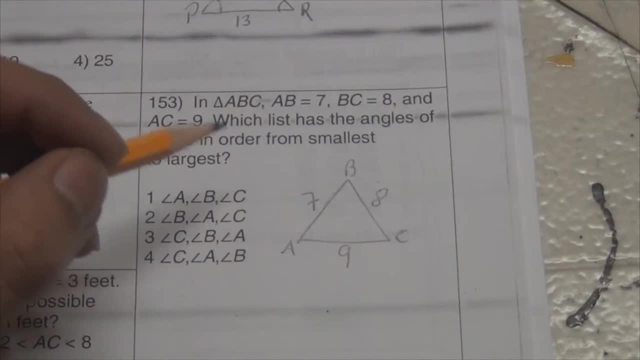 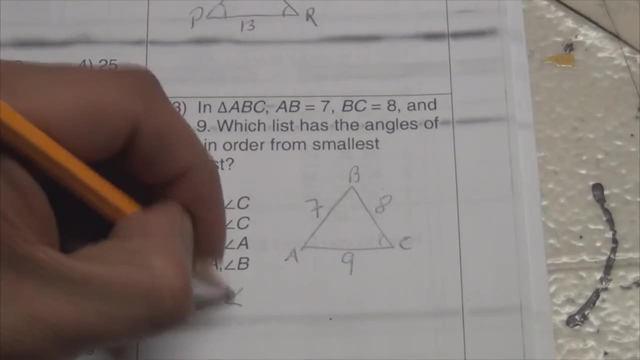 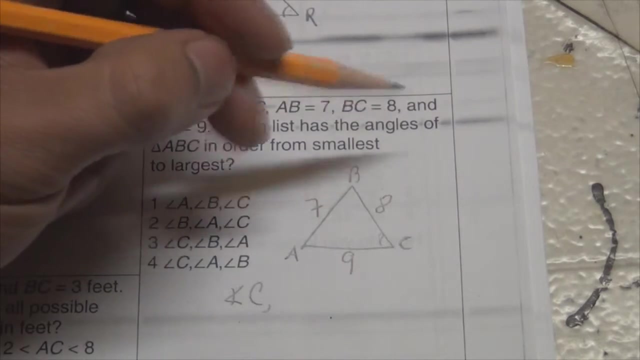 Smallest to largest. sure, What is the smallest angle? Well, this is the shortest side, So the smallest angle is C. The next smallest Angle is in order is what? Well, the next shortest side is B, C, which is 8.. 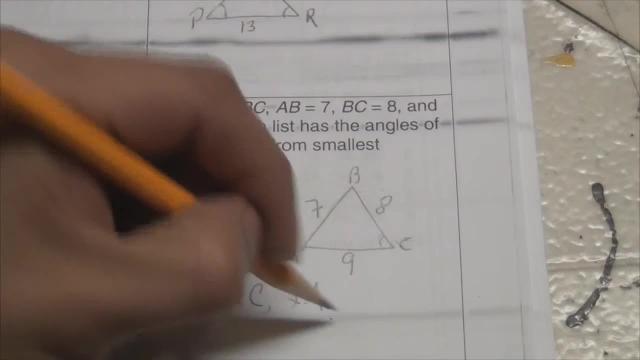 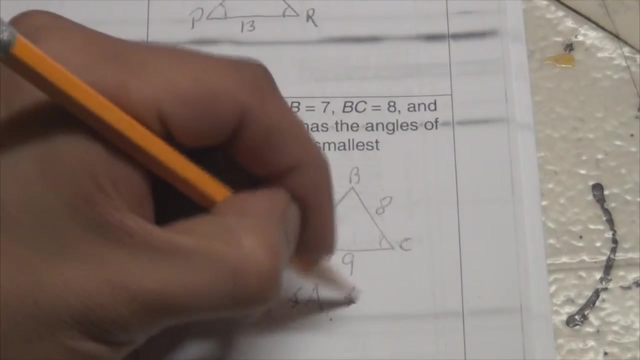 So opposite to 8 is angle A And of course the largest, well the longest side is A, C. So opposite to A, C is B. So now we'll look at the choices C, A, B. 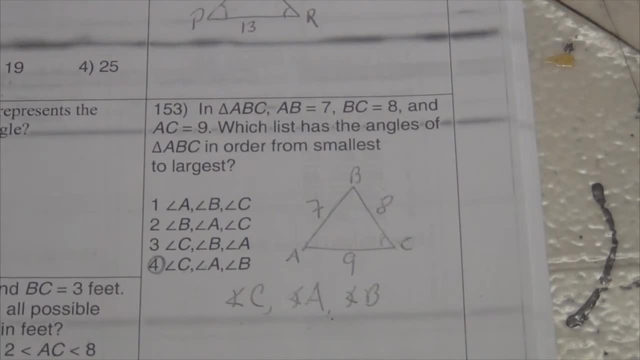 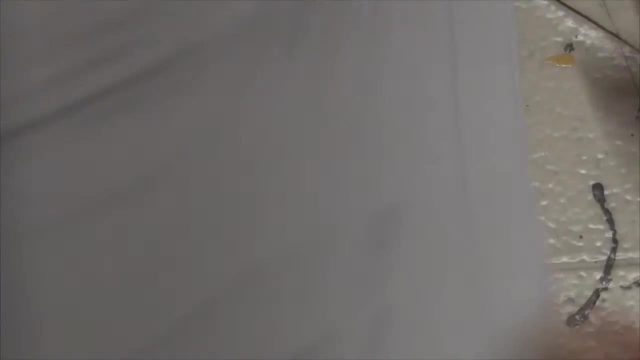 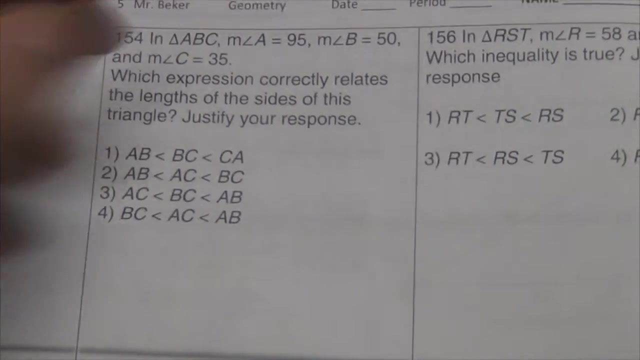 Which one has C A B, C A B right here. Boom, And that's your answer. Okay, let us move on. Let's see what we got here. All right in triangle ABC, once again visual. 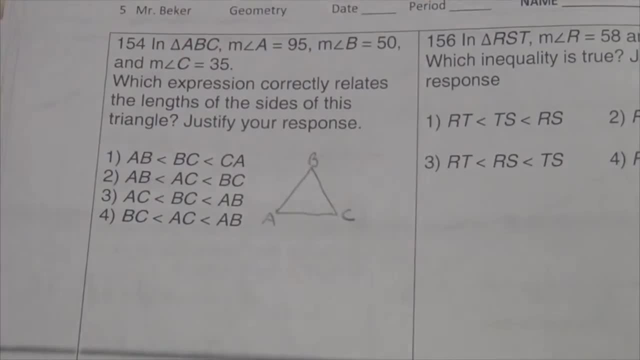 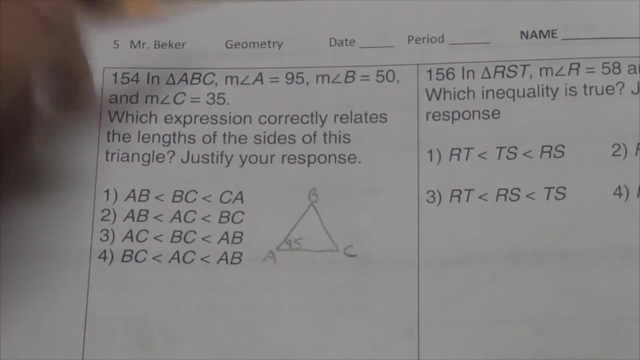 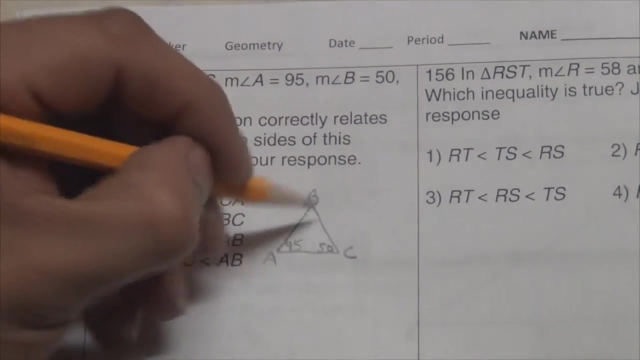 Okay, A, B, C. Now. angle A is 95.. Okay, Angle B is 50.. See how I'm putting the numbers inside. Now, if you cannot put it inside, then you make a reference arrow pointing that that. 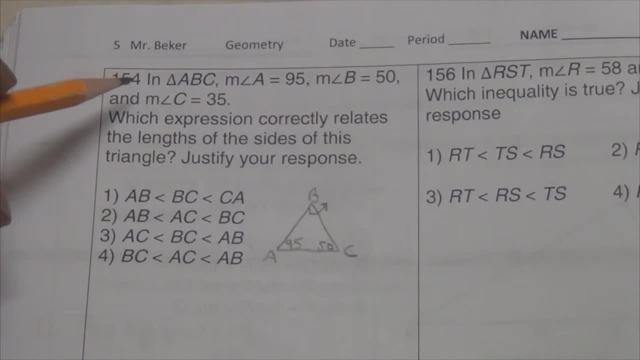 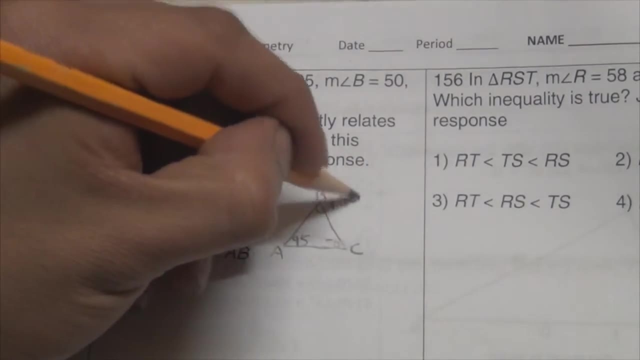 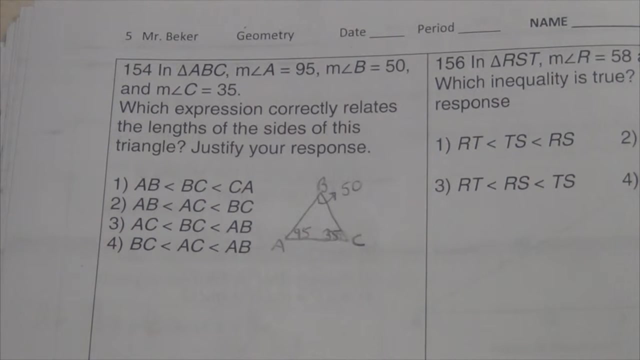 is an angle, So angle C is wait. oh my God, I'm in a mistake again. Angle B is 50.. And angle C is 35.. Okay, Now, once again, if you catch me in one of my mistakes, I'll give you two points. 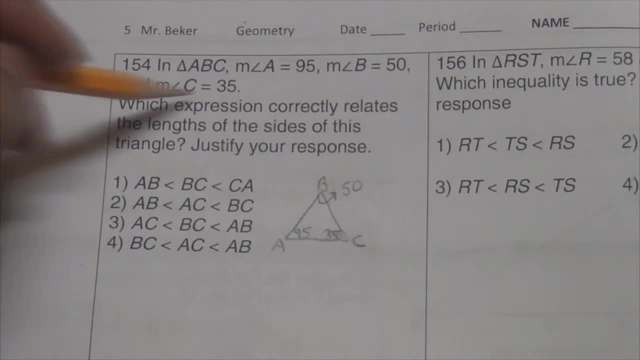 All right then. So now, what do they want? What do they want? Which expression correctly relates the length of the sides- okay, of the sides of this triangle, Justify your response, And then they give us some choices right here. 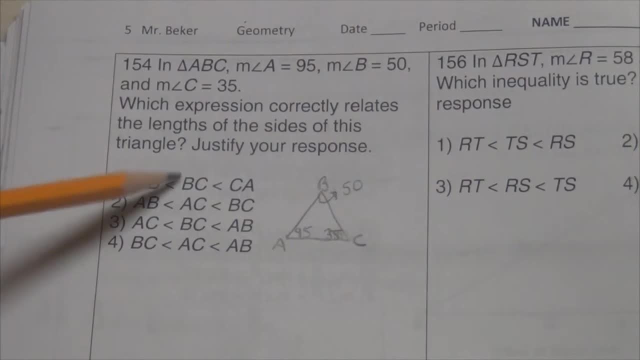 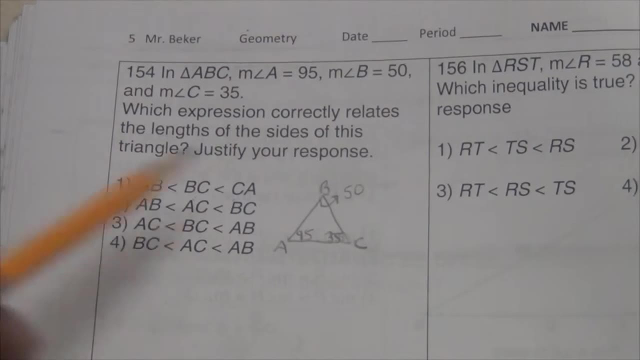 Now notice that the symbols here, the inequality symbols, are less than Less, than Meaning that this is smaller than this one and this is smaller than this one. Oh, so I'm going from smallest to largest, Okay, And we're talking about sides. 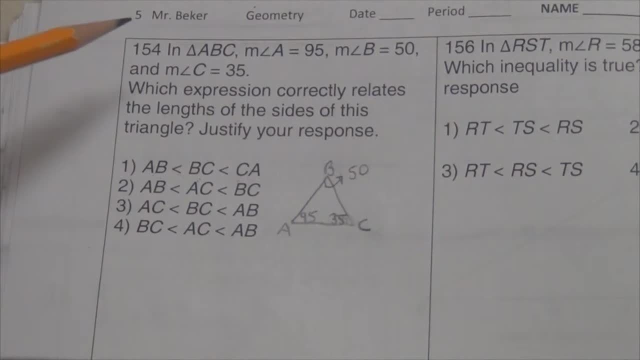 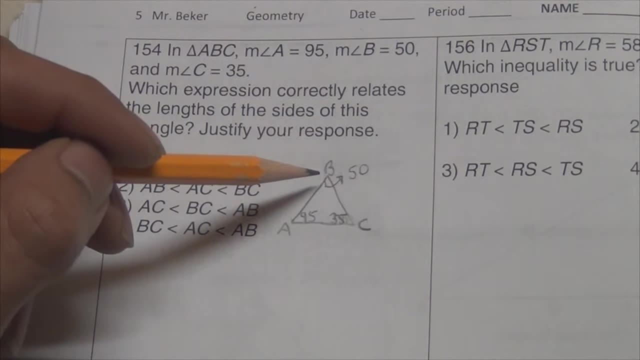 So let's see Which one is the smallest side. Well, The converse is also true. If opposite to the longest side is the largest angle, then opposite to the largest angle is also the longest side, and vice versa. Okay then. 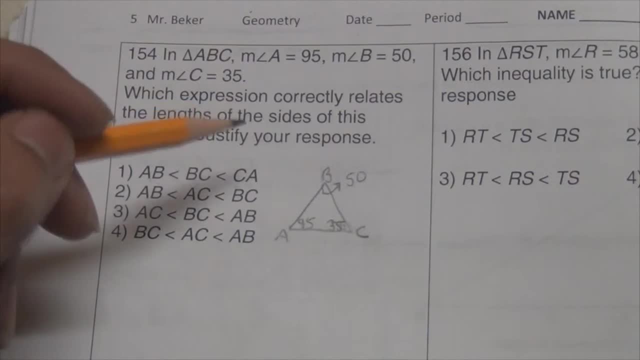 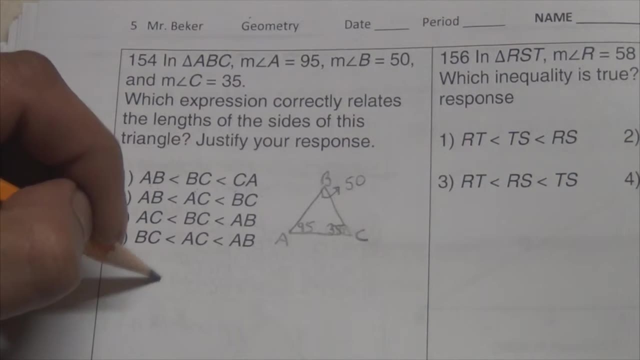 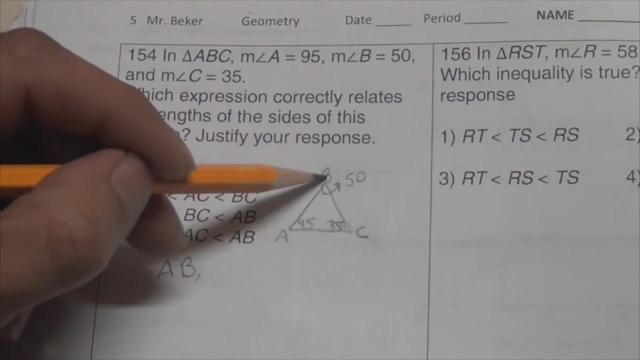 So let's go from smallest to largest. Which one is the smallest side right now, Before I write it, One point, Five seconds. A, B, Very good. What is the next smallest? Well, right here I have an angle of 50, so the next smallest is A, C. 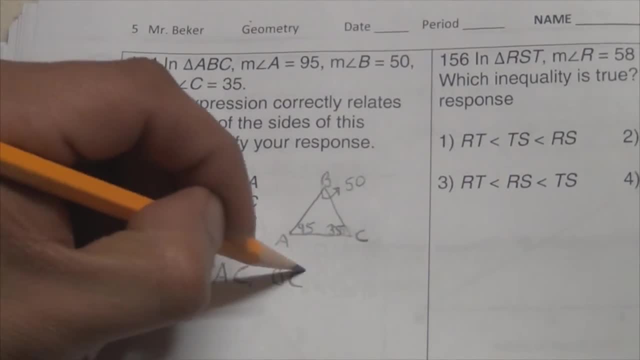 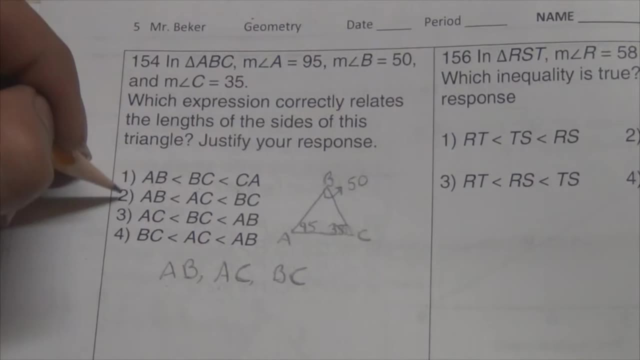 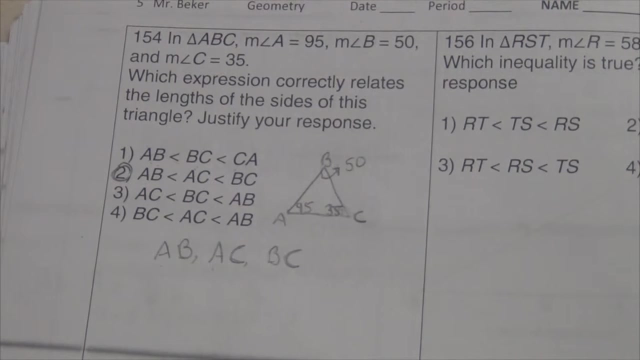 And then the largest would be B C. So we got A, B, A C and B C. Which one is the answer? Ooh, Lil Wayne, As long as my girls love me, my girls love me, my girls love me. 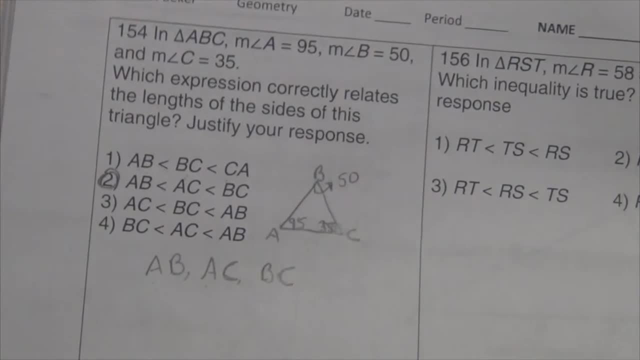 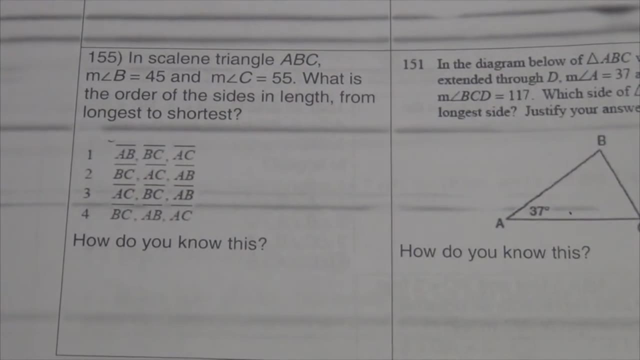 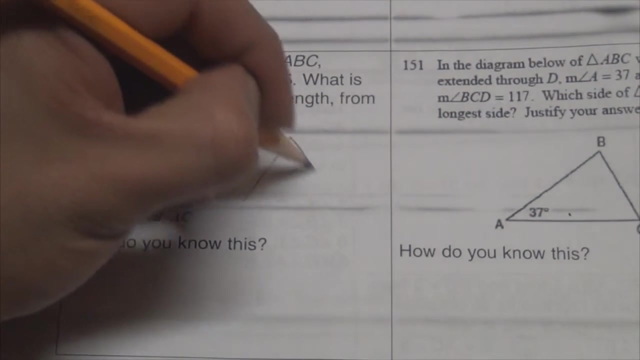 Oh, with no makeup, she's a 10.. She's the best with the brains, Okay, So let us move on to this one. All right, that's it. You can actually do this on your own, but just remember, it's always easier if you have a reference, a visual. 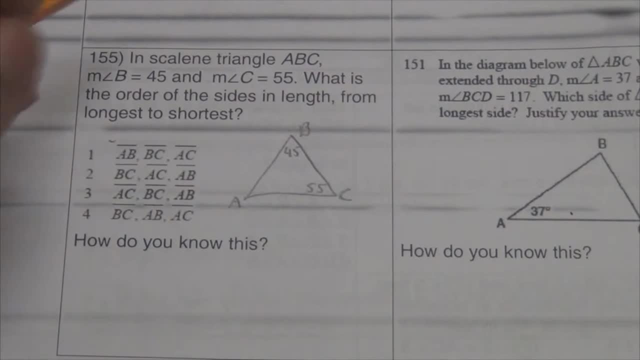 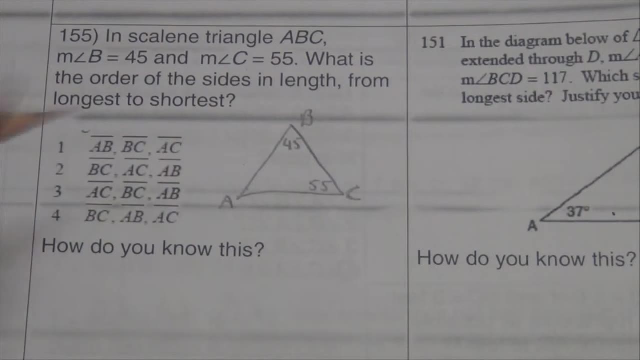 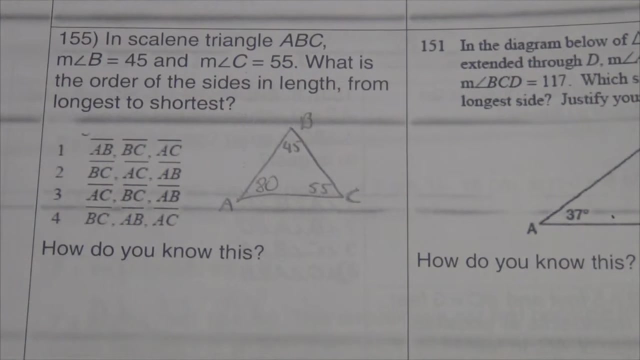 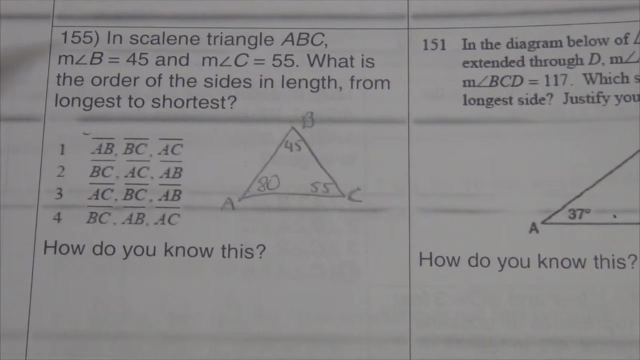 Or show them again whenever you make it that way, they totally won't broke their memories, Okay. So this is the last one. How do I get this? Well, you tell me. Okay, Okay, Okay, Okay, Okay. 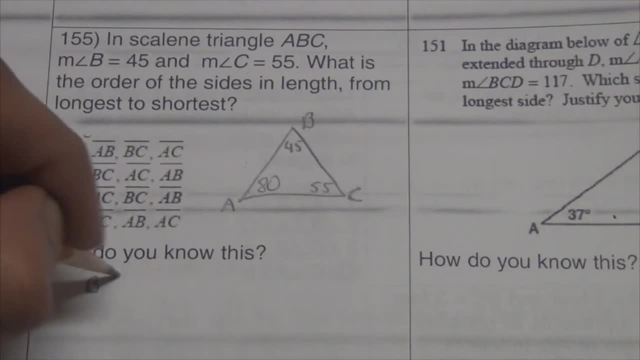 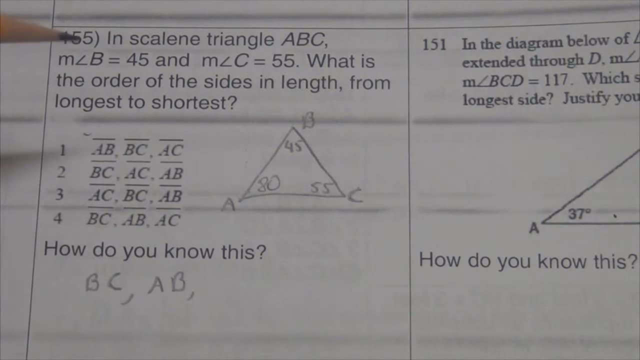 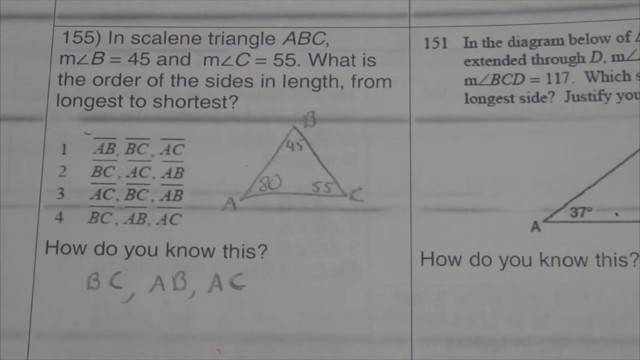 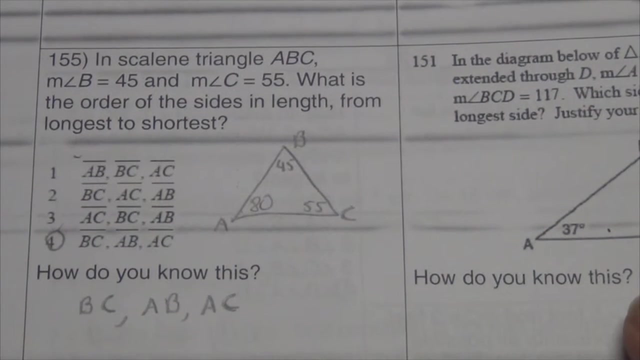 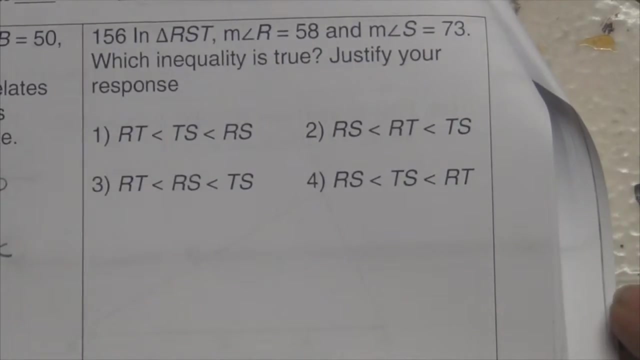 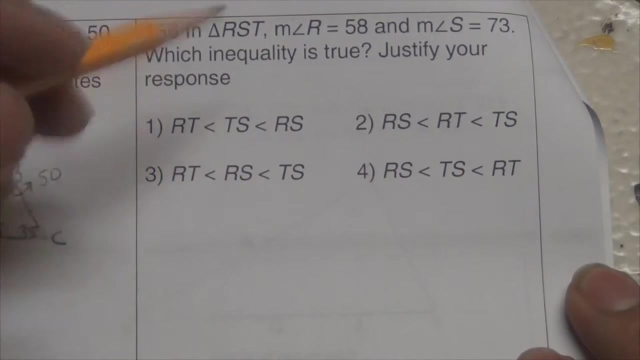 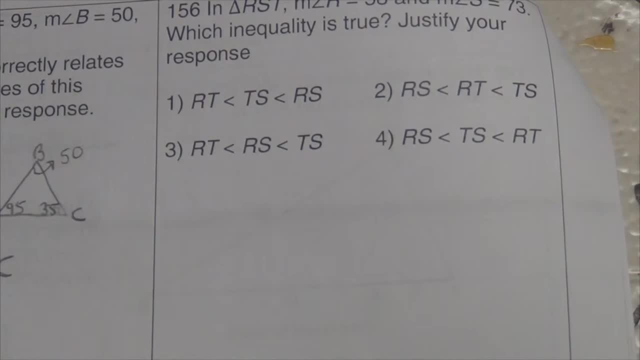 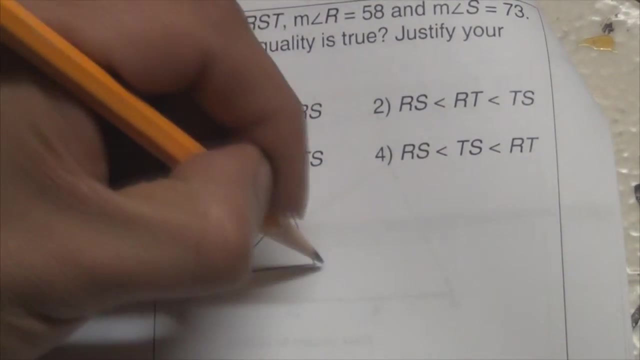 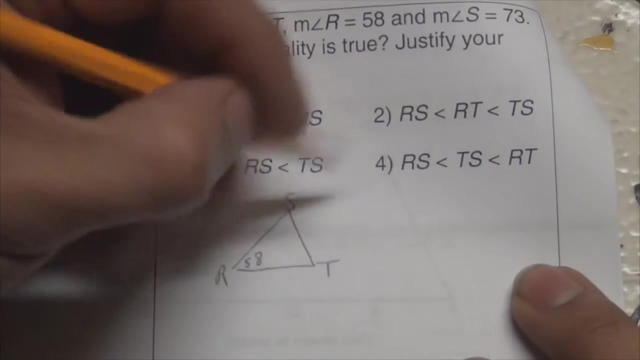 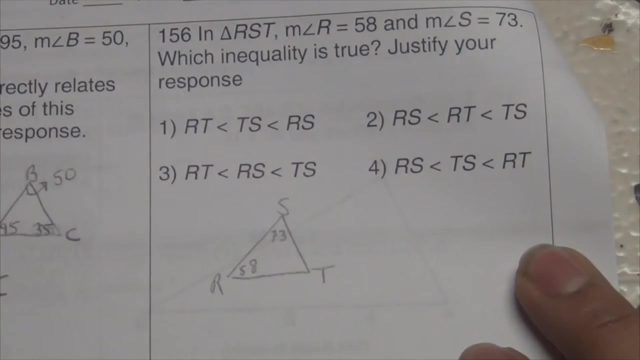 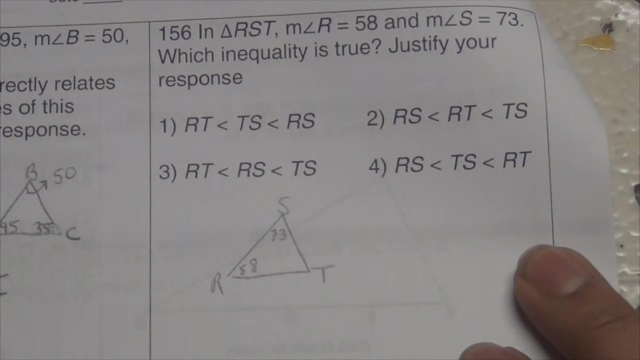 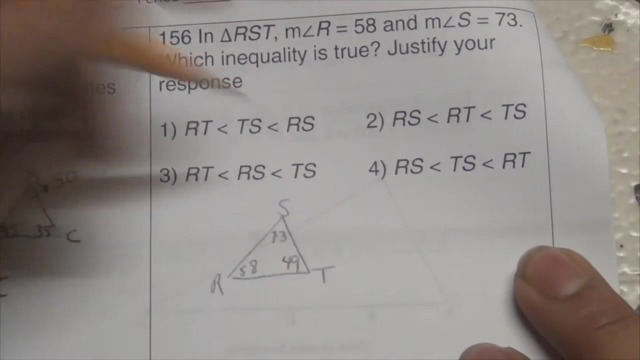 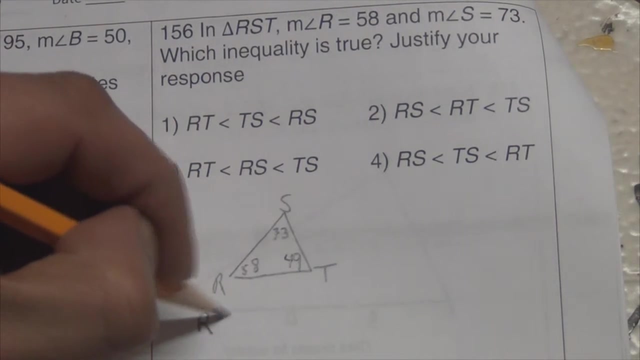 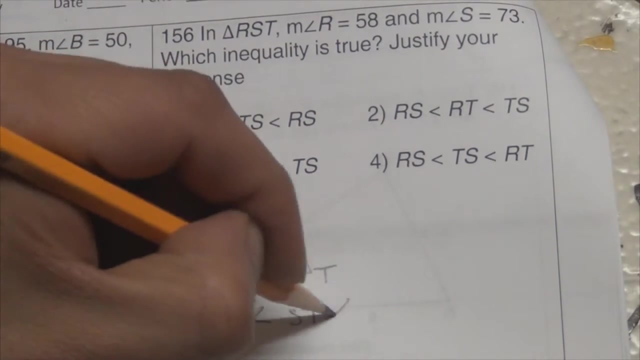 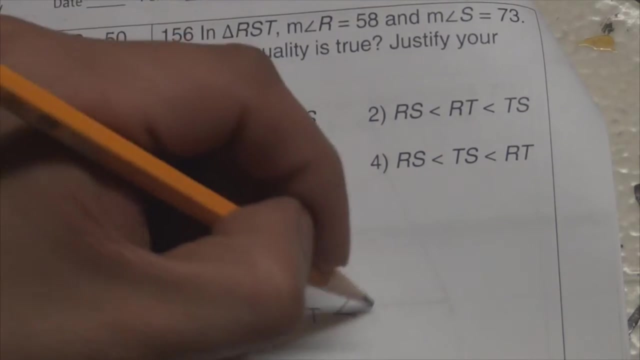 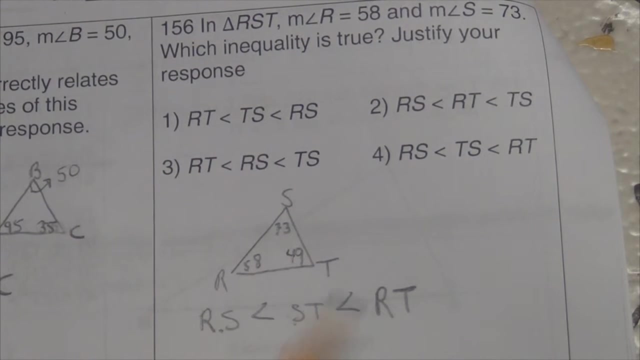 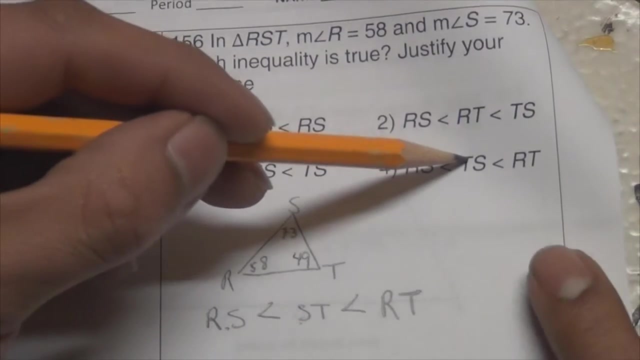 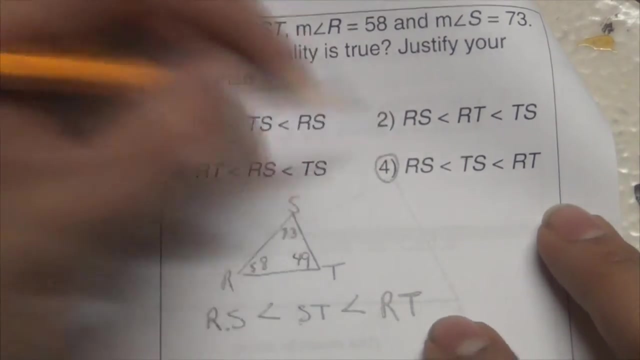 answer this question: you, you, you. you is smaller than ST and ST is smaller than RT, so you make your selection. Now, this one says RS, this one says TS, so TS and ST should be the same thing. Okay, okay, okay, Becca, I'm sorry, I'm sorry, Never doubt me, son. Never doubt me If you. 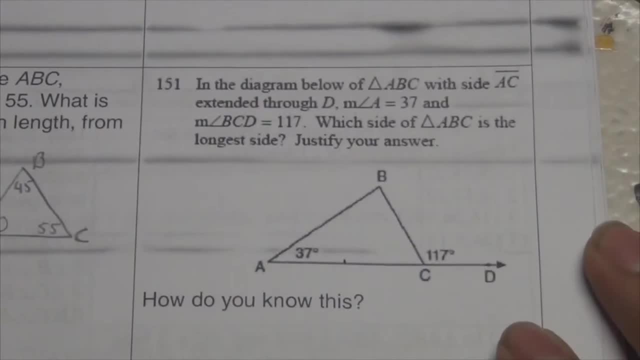 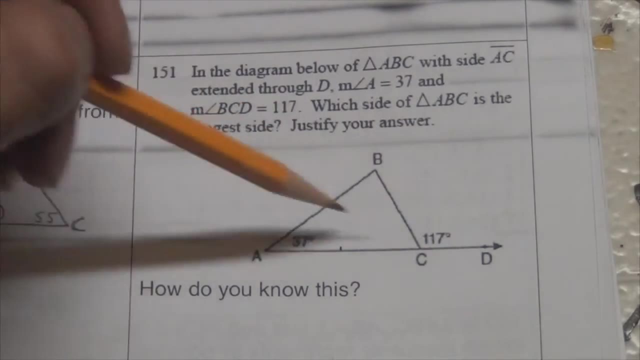 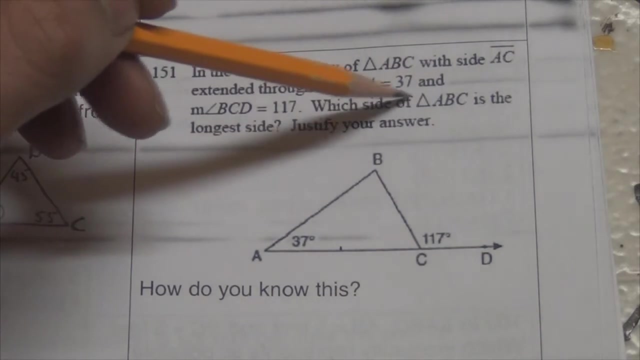 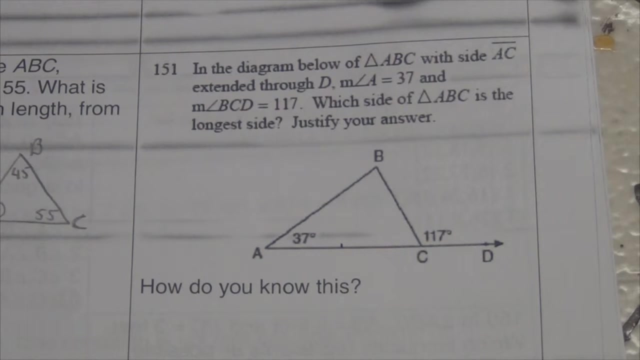 doubt me. you get this In the diagram below of triangle ABC. oh, at least they gave me the diagram. okay, What do they want? Which side of ABC is the longest side? Wow, which side is the longest side? Therefore, I have to utilize the external angle theorem of triangle ABC. 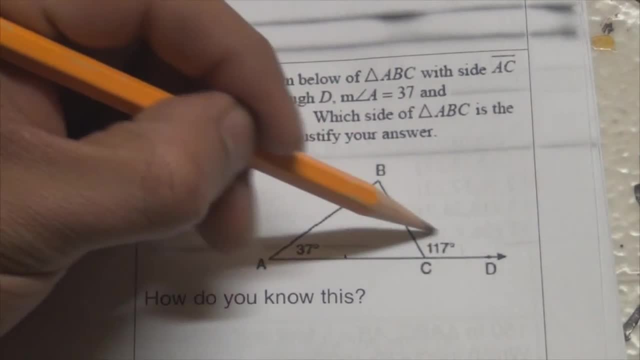 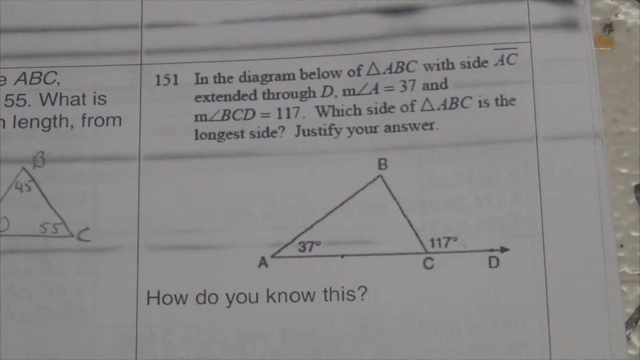 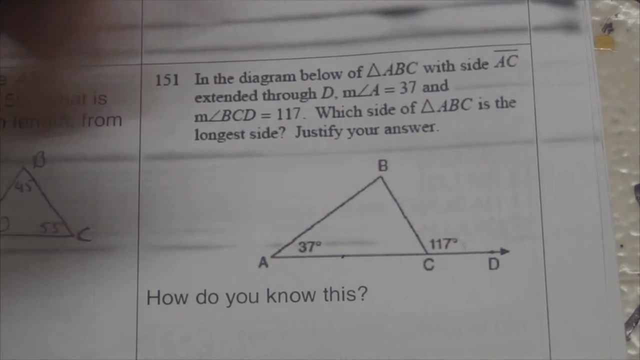 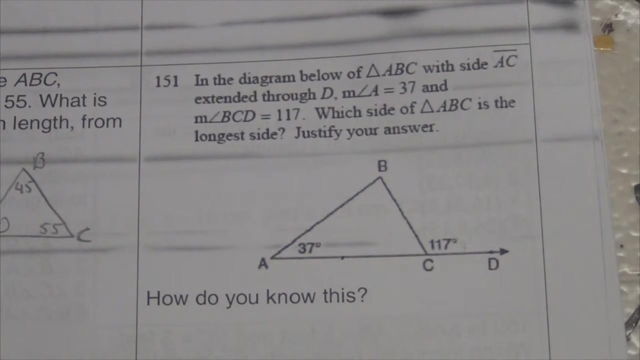 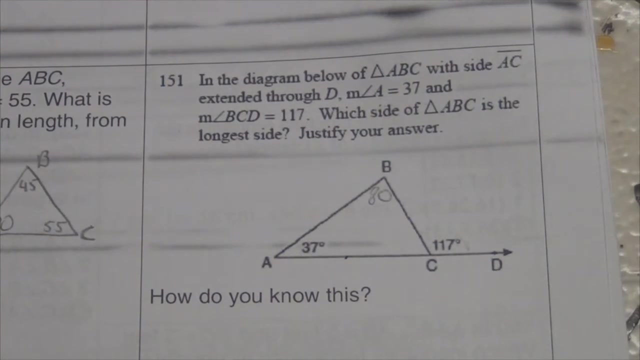 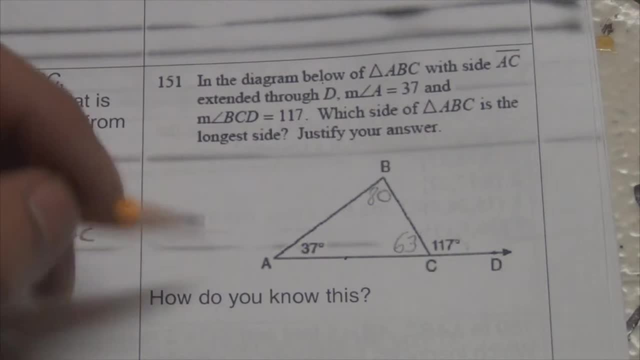 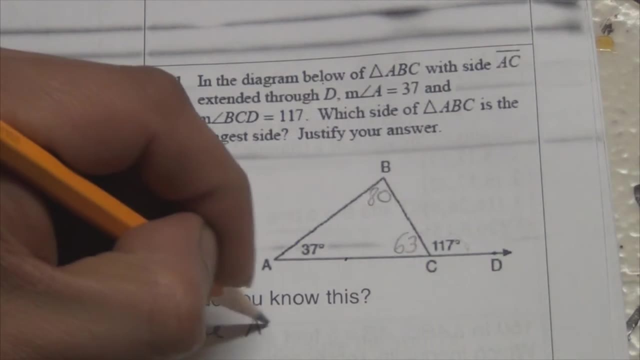 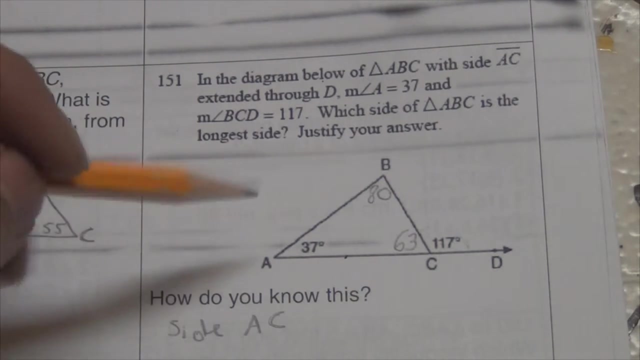 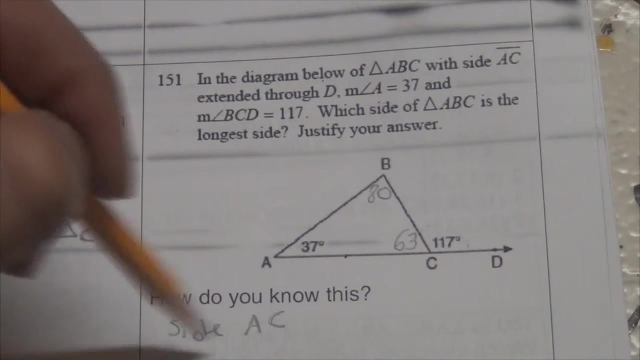 Okay, How do I know this? Well, because of the Triangle Inequality Theorem, which states that. What does it state? Wait, hold on a second. Oh yeah, I know how to justify this. So how do you know this? Easy, Because first I use the Triangle Inequality Theorem, which says that: 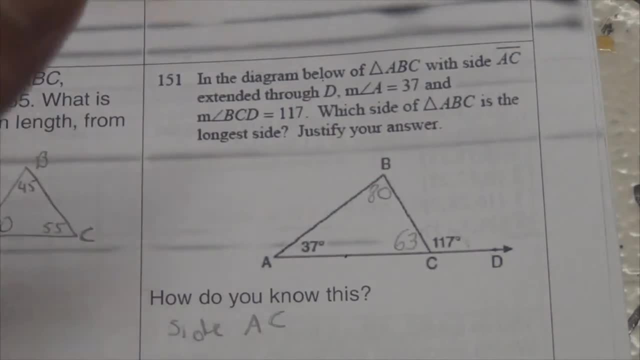 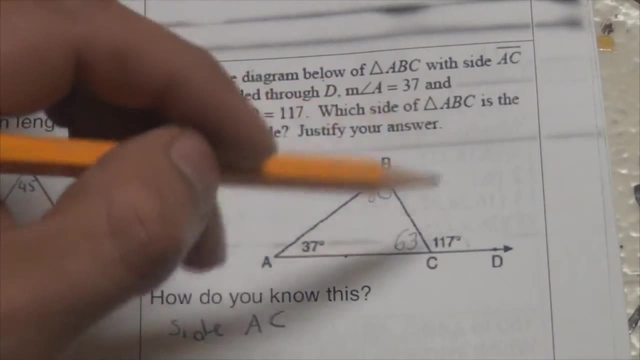 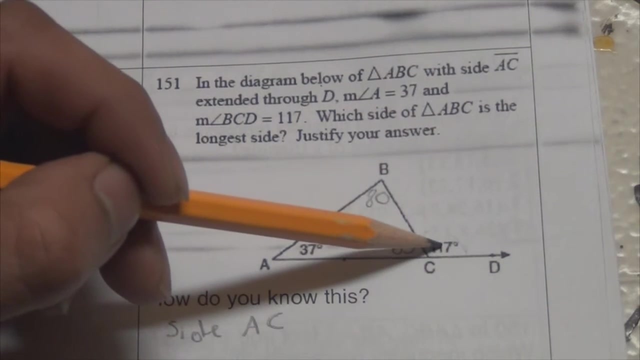 What? Triangle Inequality? No, no, no, I'm sorry, I use the- Oh, external angles of a triangle. Damn, I've been recording so much that I'm losing myself. Okay, so the External Angle Theorem says that the sum of an external angle is equal. 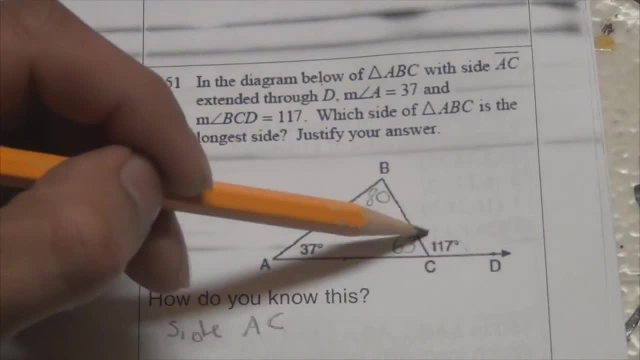 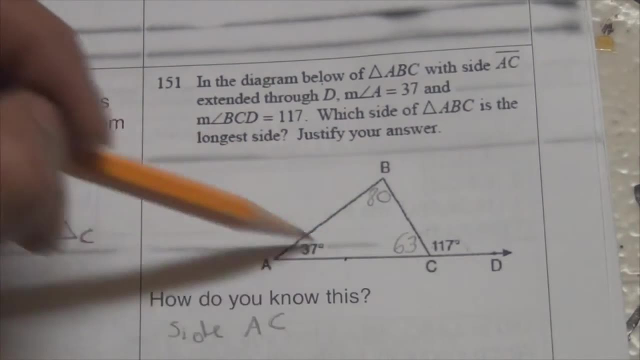 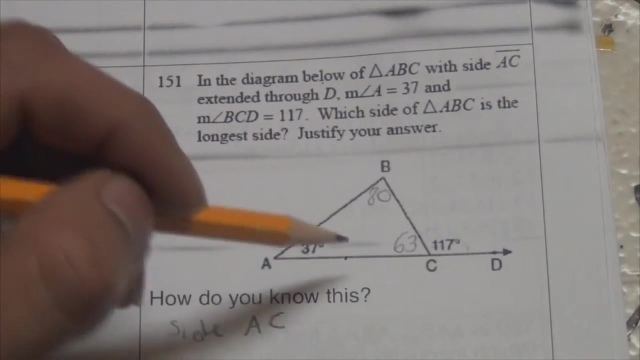 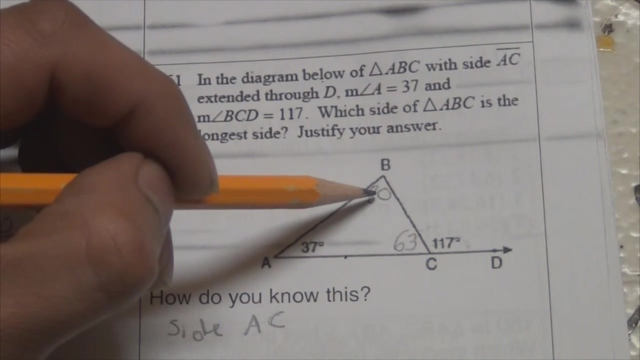 I'm sorry. Oh, the measure of an external angle is equal to the sum of the two non-adjacent angles. So that's how I figure out the measure of all angles in a triangle. Then, then, okay, I used the theorem that says that opposite to the largest angle is the longest side. 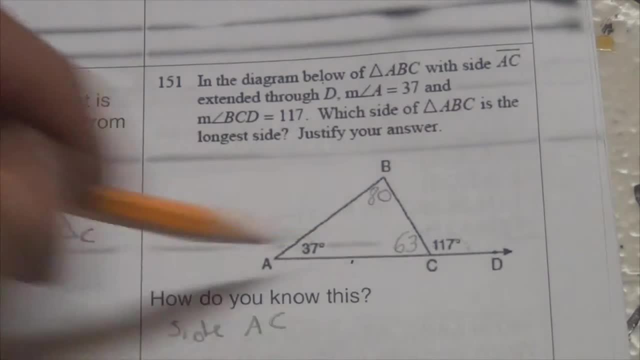 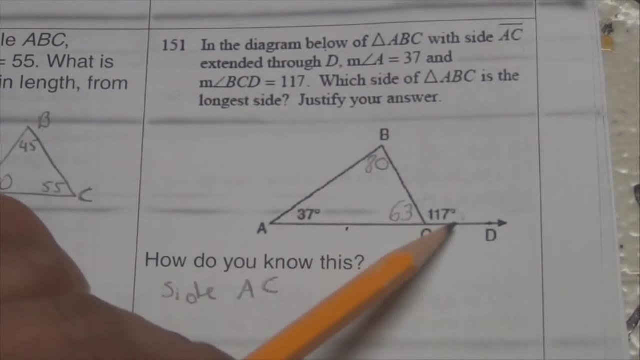 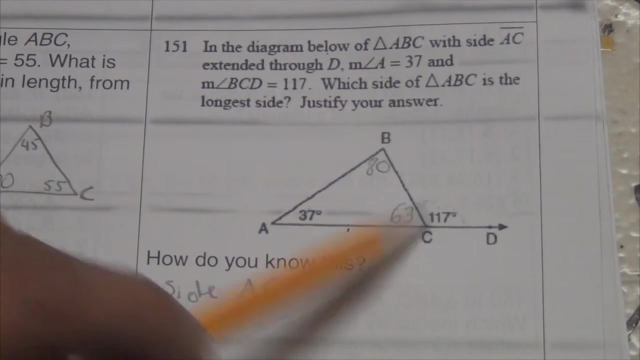 Oh, So that's how you knew that AC was the longest side? Yes, And that's how I justified my answer. And you know what? Let me rephrase this again. First, I used the External Angle Theorem of Triangles, which says that an exterior angle in a triangle is equal to the sum of the two non-adjacent angles. 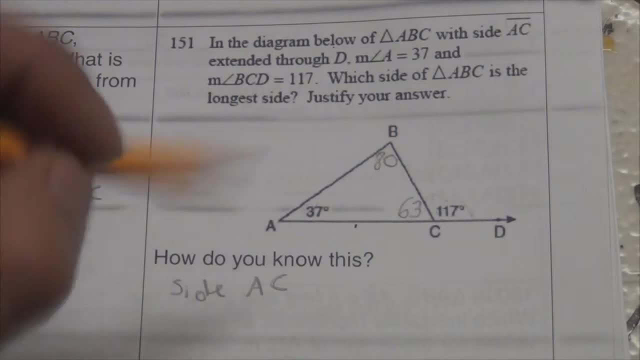 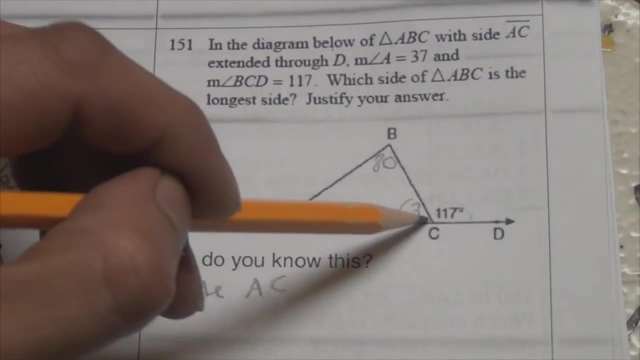 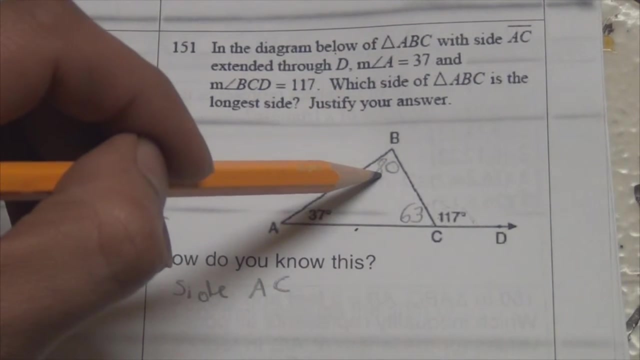 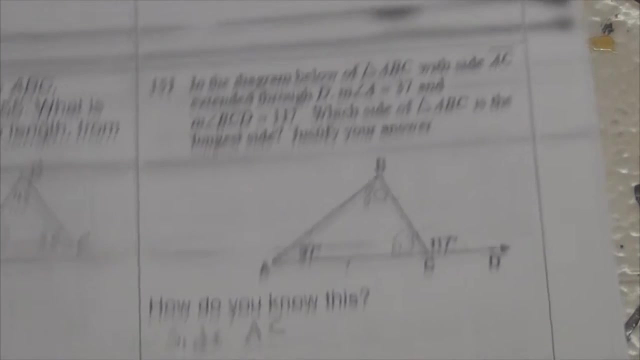 And then I remember that there's a theorem that says that, Oh, Oh, An angle opposite to the longest side is the largest, and a side opposite to the largest angle is the longest. Oh, I got it. Okay, Damn I. just I just spaghetti myself. I tangled myself into this. 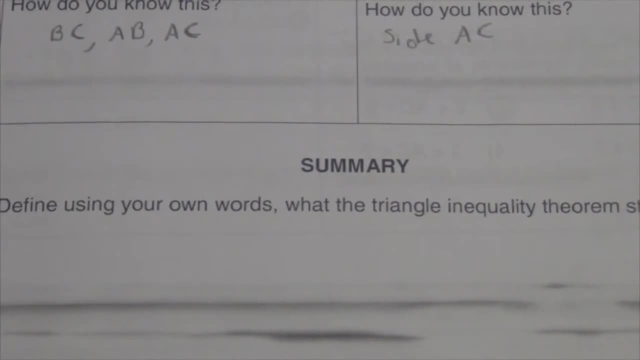 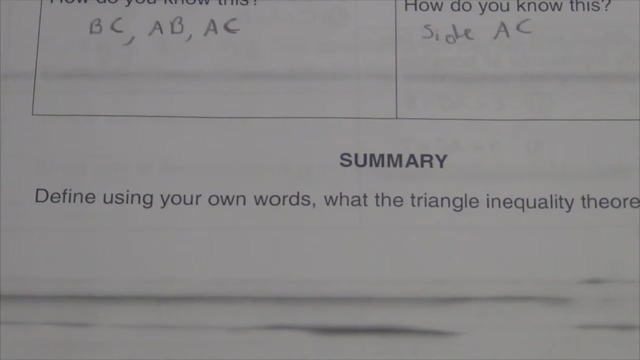 Alright, so what does it say here? Define, using your own words, what is the triangle inequality? What does the what the triangle inequality theorem states? It states that the sum of any two sides Of a triangle Is greater than the length of the third side. 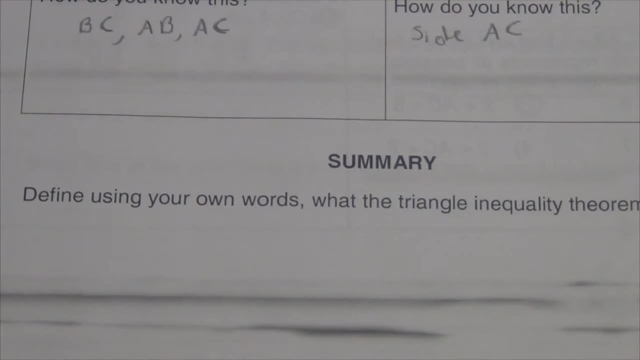 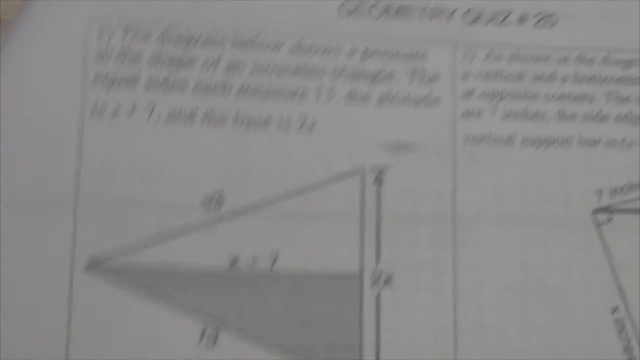 I don't have to write it down. You already have it in the mini-lesson, so just refer back to the mini-lesson so you can write down your summary. Alright, Good, Alright. Quiz number 25.. Wow, we've been through this already. 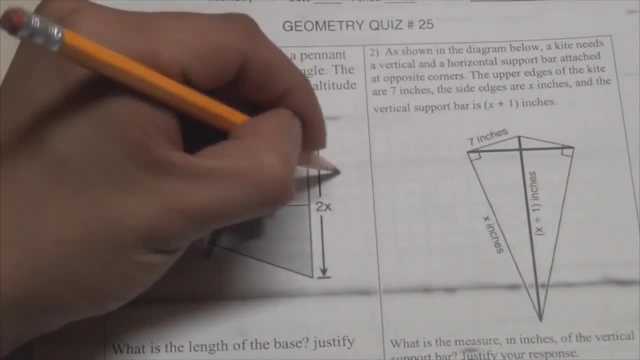 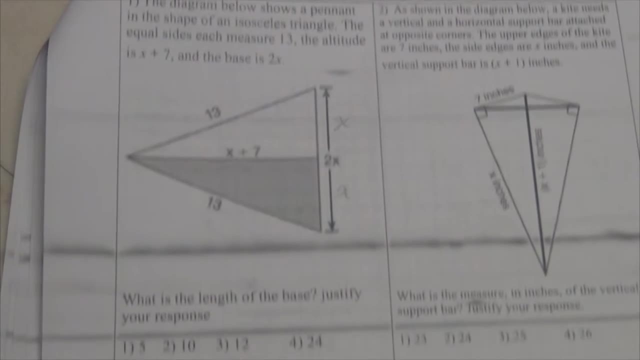 Here they want the length of the base. This is an altitude. So this is x, This is y, This is y, This is x, This is x is X, Alright, Alright. so now I'm going to use Pythagoras, because this is the right triangle. 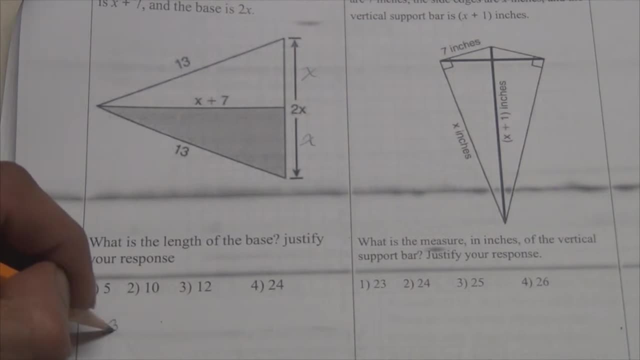 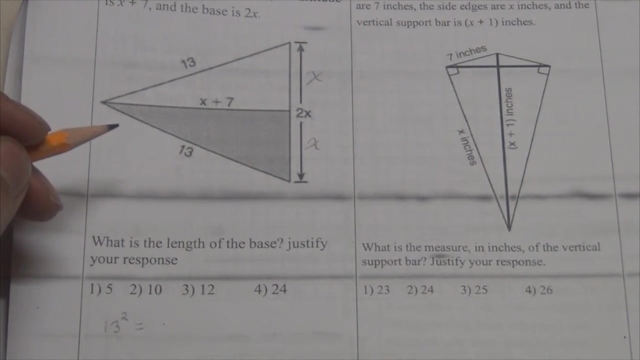 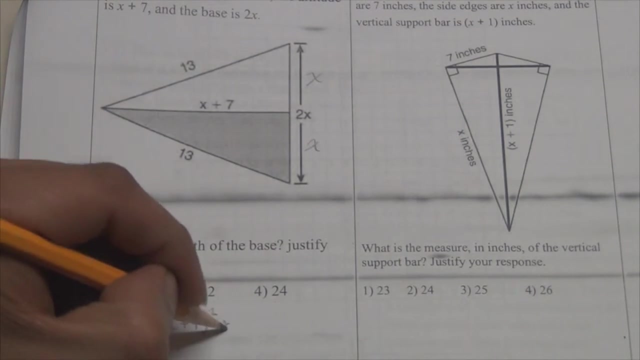 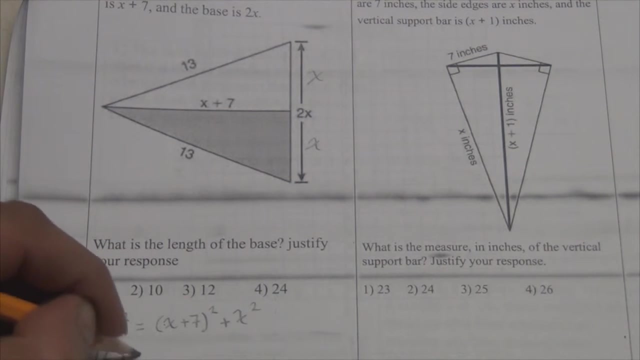 So I'm going to say, okay, the length of the hypotenuse square is equal, okay, to A square plus B square. Okay, so A square is going to be X plus 7 square plus the other leg plus X square. Alright, so 169 equals. and then what is X plus 7 square? You are squaring. 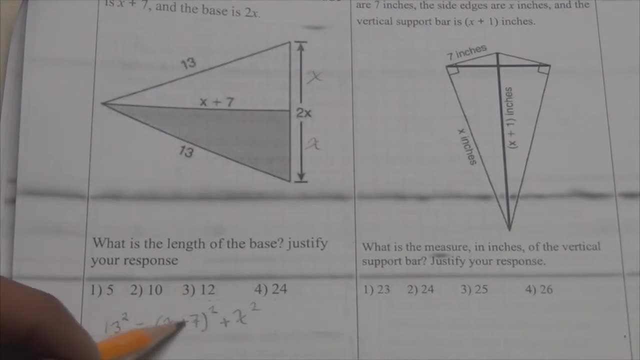 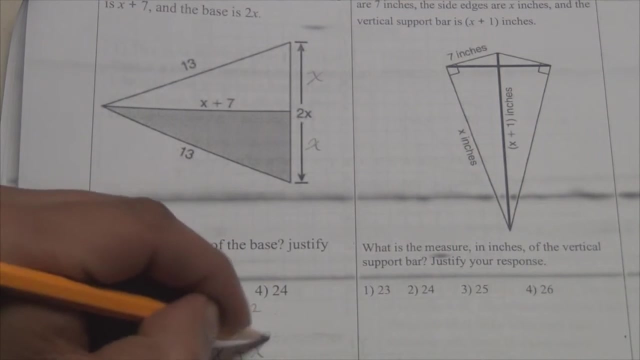 a binomial. Okay, that means you're multiplying this by itself. So how do you do that? Easy Square, the X. get this together, 7X, right. 7X times 2, that's 14X, and then plus X square. 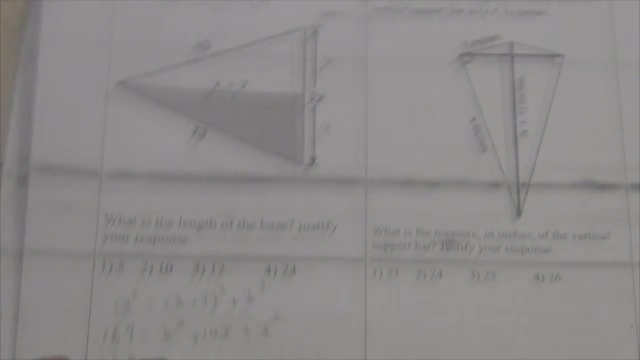 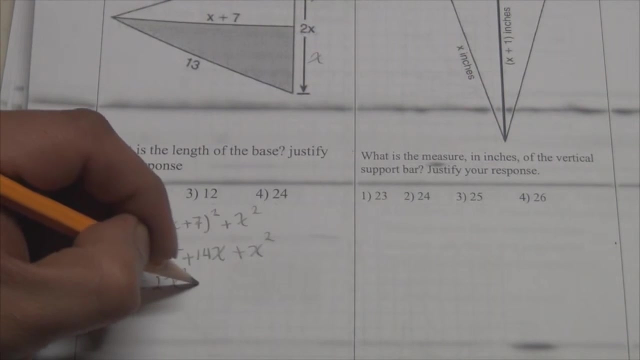 Then you're going to combine like terms, So you're going to have 169, sorry, 169 equals X square plus X square is 2 of this, so 2X square plus 14X. Then we know that this is a quadratic equation, because I did not cancel. 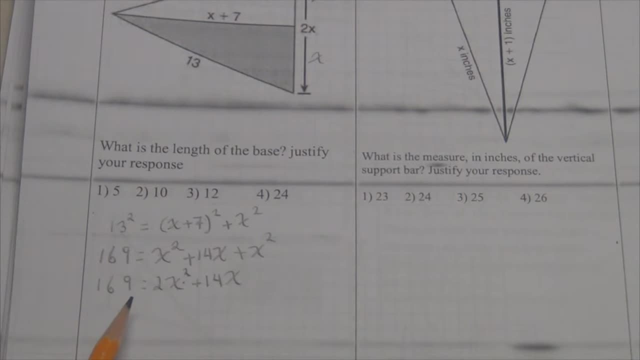 anything. What's up? What's up? Nothing. Okay, so now we're going to equal one of the sides to 0, because this is a quadratic equation and quadratic equations should be equal to 0.. Okay, so subtract 169.. 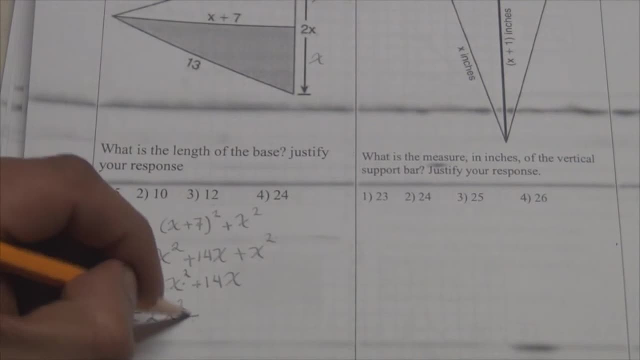 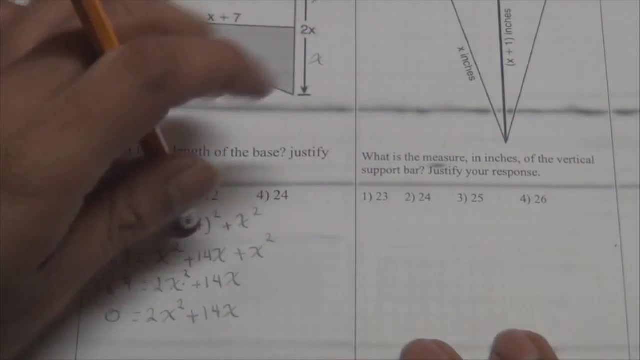 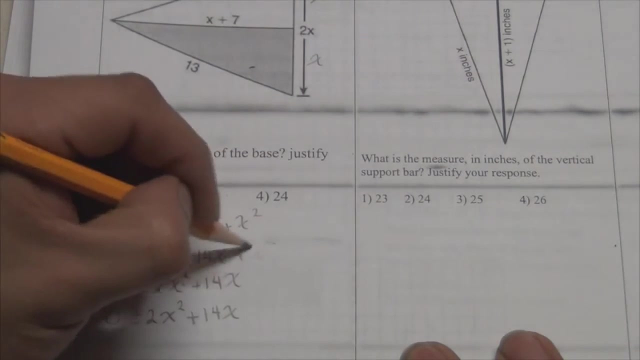 169 from both sides. Wait, I missed something here. What did I miss? Oh gosh, Hopefully you caught it and you corrected me. I forgot to square the 7.. So this is 49, and then plus X square 49, okay, plus X square Oh. 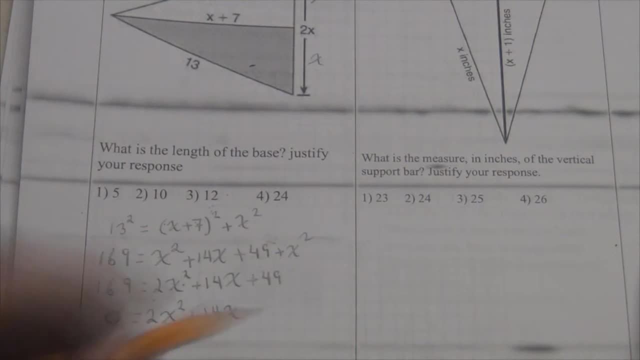 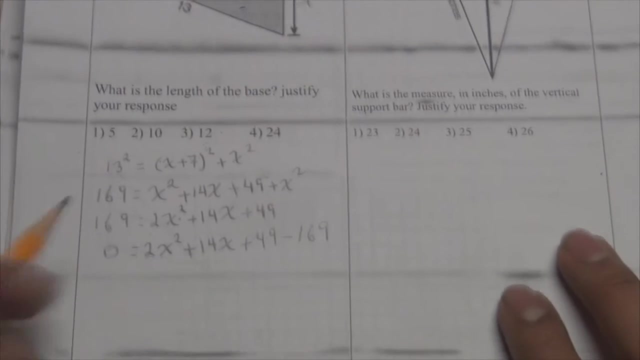 of course what this is, So thisided it out now Here. this is funny why it's hard to figure it out. So I subtract barely: wasn't over 1!. Okay, I want to make it a little bit easier with a calculator. Then what do I have on? 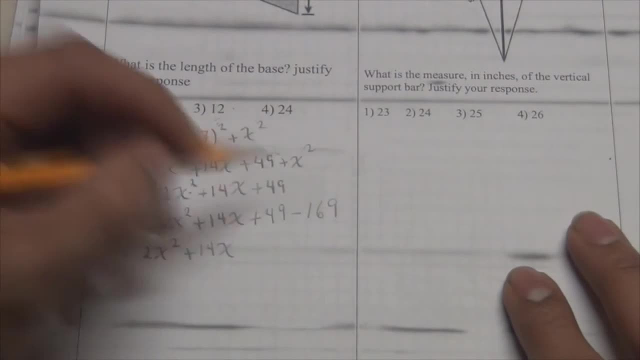 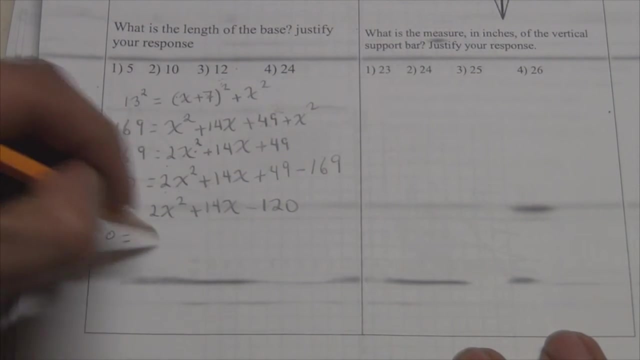 my exactly purchase manager. Look, let me just 후�. let's do a little bit of a math test. let's say: Mersers Hardwarextractor 1,, 6,, 2,, 3,, 4,, 5.. 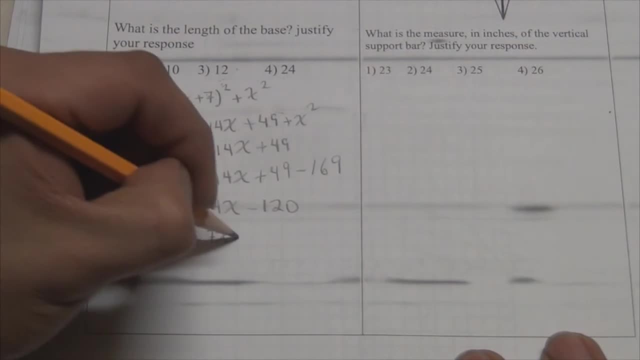 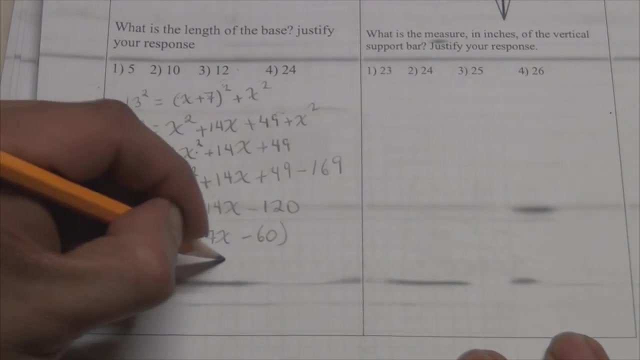 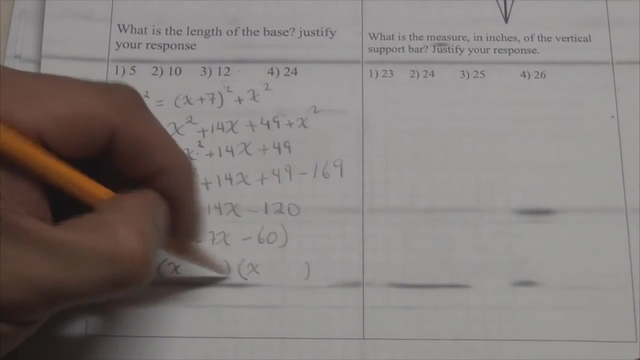 I, x, 2.. x squared plus 7x minus 60.. Then we continue with the factoring. So we open the parentheses And we say: factors of x squared is x and x Factors of 60,. well, we already know it was 12 and 5. 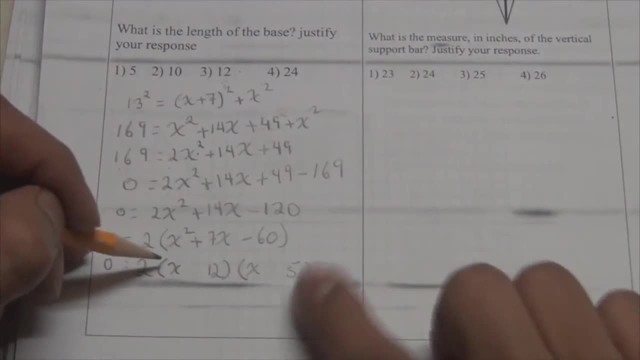 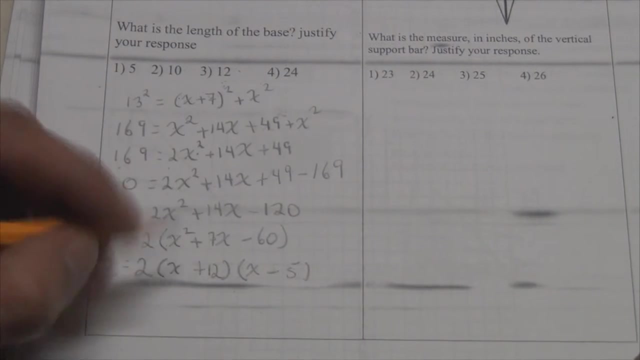 because 12 times 5 is 60. I do the smiley face, so I get 5x and 12x. How do I get 7x? Make this positive, make this negative, okay, And we don't know. 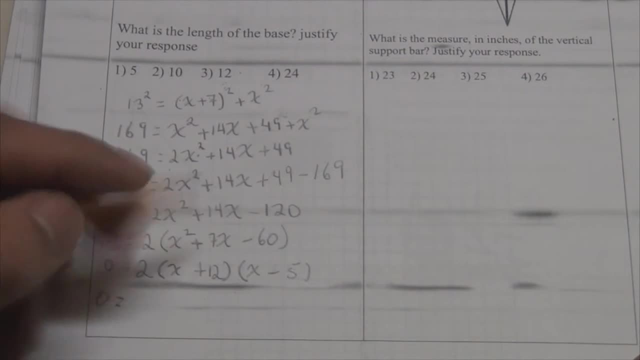 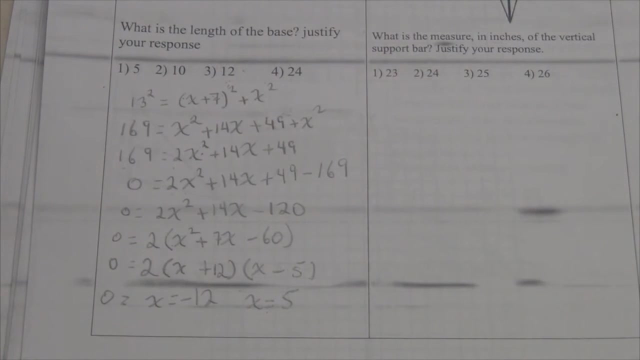 So now we have the solutions. What number plus 12 is 0? x equals negative 12.. What number minus 5 is 0? x equals positive 5.. So we're going to use the positive value of this and we're going to substitute it into our base. 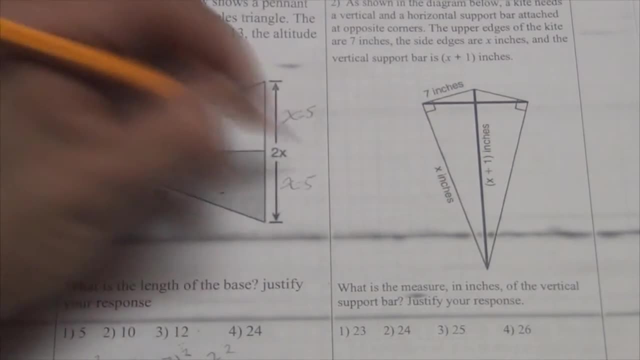 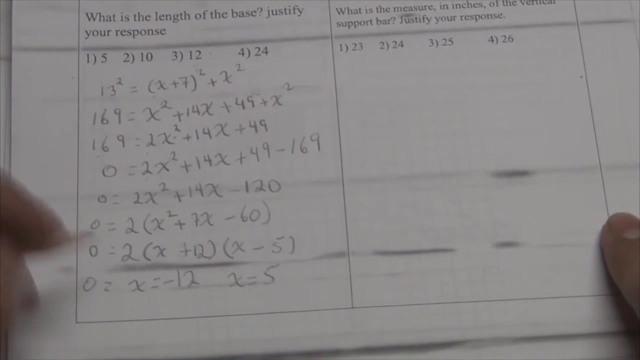 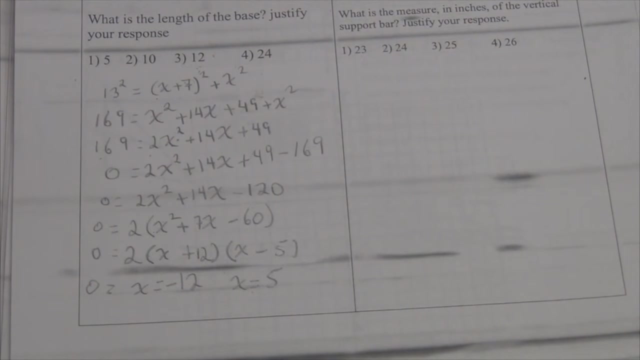 So this is 5 and this is 5.. So the total value of the base is 10.. So please write it down, Write it Like the value. Okay, the length of the base is 10, whatever units they're giving you. 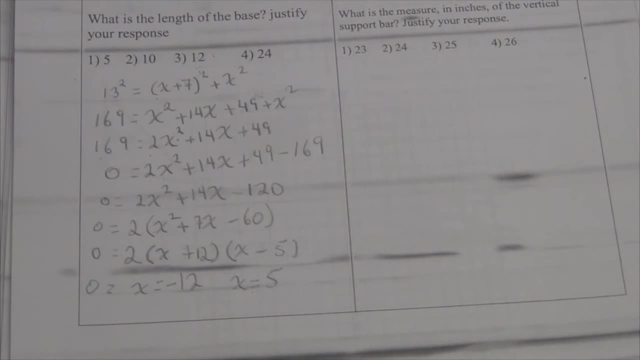 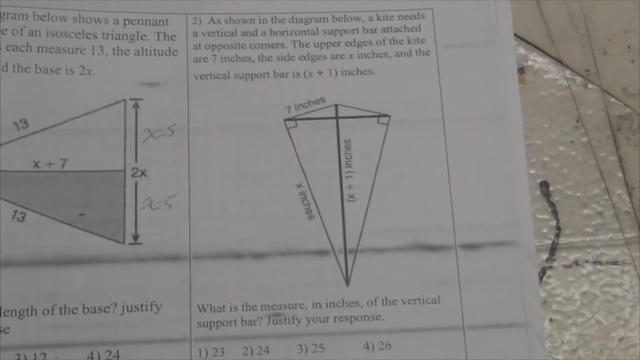 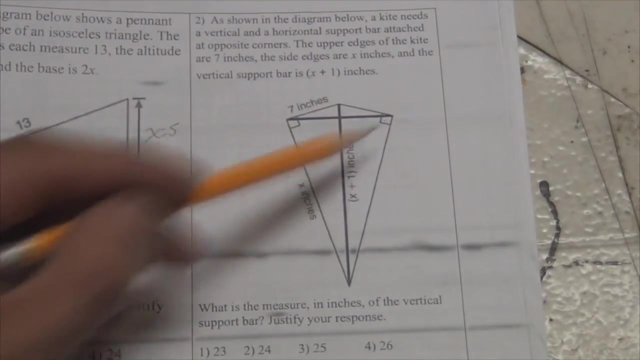 Okay, Oh God, I'm tired. All right Now, this problem, right here. Okay, so it says a kite needs a vertical and a horizontal support bar. This is the vertical bar. This is the horizontal bar. okay, Attached to opposite corners. 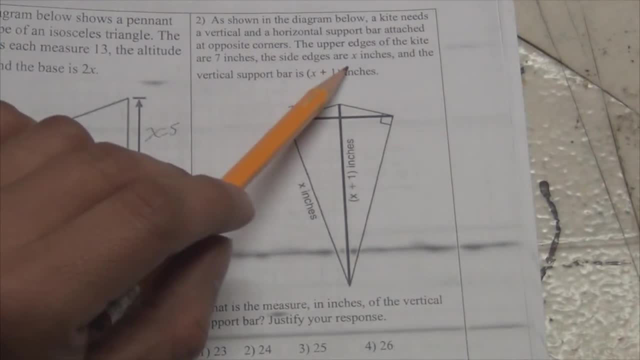 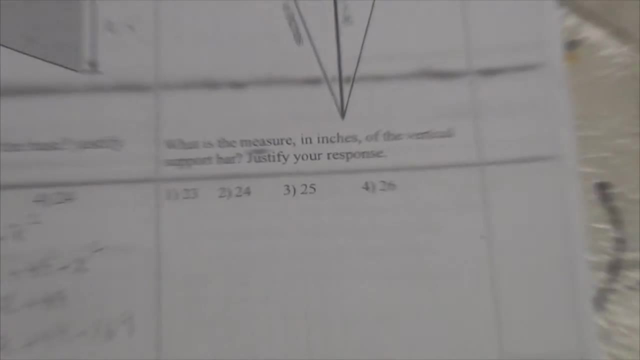 Okay, Okay, Okay, Okay, Okay, Okay. So the height are 7 inches, The side edges are x inches and the vertical support bar is x plus 1 inches. They want what They want. what is the measuring inches of the vertical support bar? 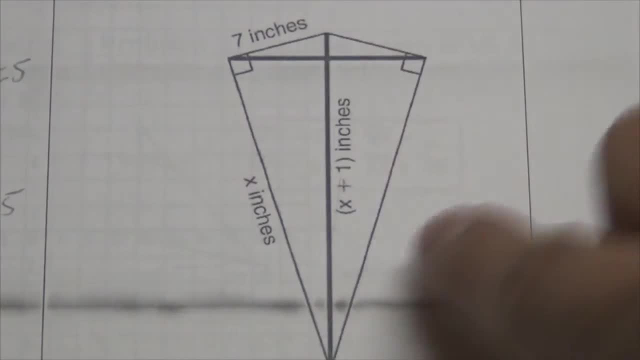 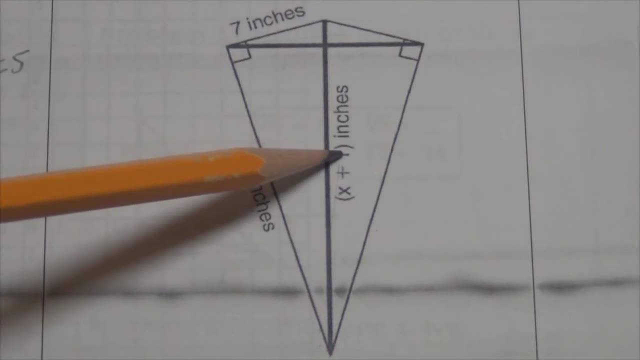 They want to know what this is Okay, so look, two right triangles, So I just need to use one of them: Leg leg hypotenuse. Opposite to the right angle is the hypotenuse. So that's what I'm going to do. 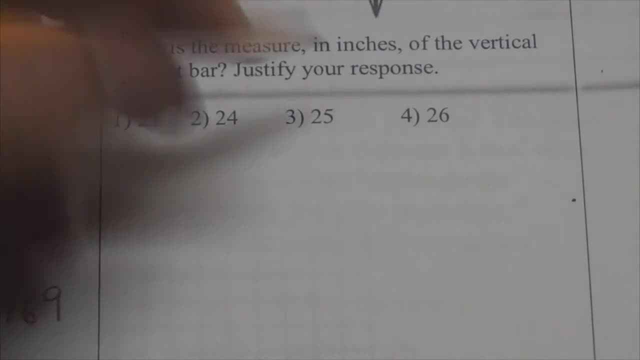 So I'm going to start using Pythagoras. So tell me What is the hypotenuse? The hypotenuse is x plus 1.. So x plus 1 squared equals to a squared plus b squared. So 7 squared plus and then x squared. 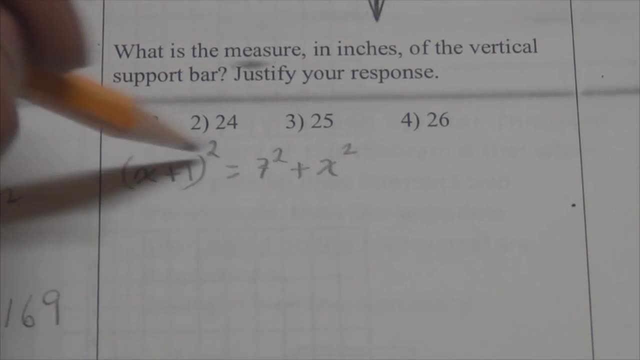 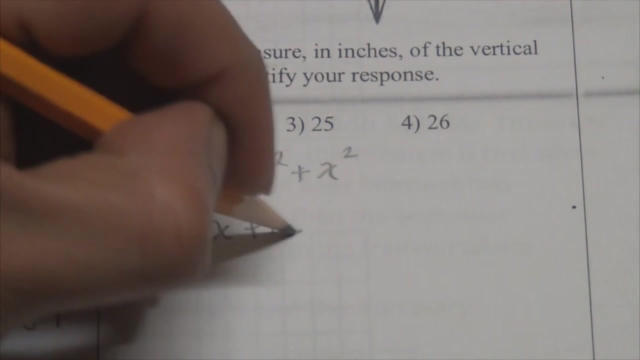 Okay, What is x plus 1 squared? You already know how to square binomials, So square this one, So I get x squared, plus Put this together and times it by 2.. So you get 2x plus 1, equaling to 49 plus x squared.